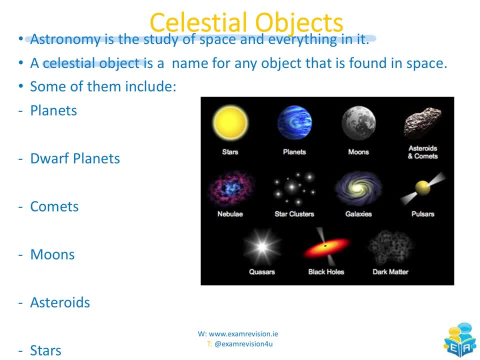 asteroids and comets. we've nebulae, star clusters, galaxies, quasars, black holes, dark matter. all of these will be examples, But the ones which we need to know for junior cycle science are our planets, our dwarf planets, our comets, our moons, our asteroids and our stars. It's vital. 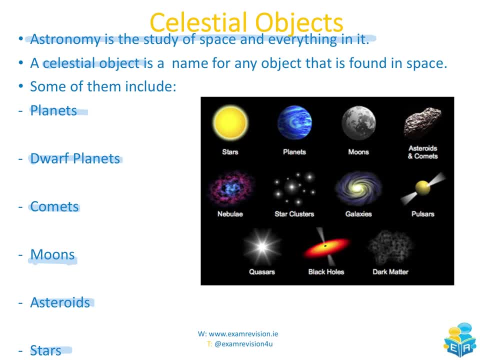 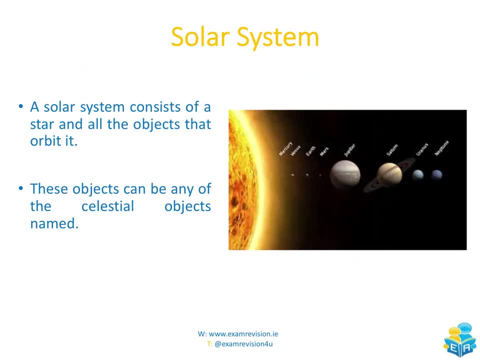 that we know all of these, and we'll be going through each one of these in a little bit of detail over the next couple of slides. Okay, so the first thing we're going to focus in on here is the idea of a solar system. So a solar system consists of a star, which, in the case of our solar system, is the sun. 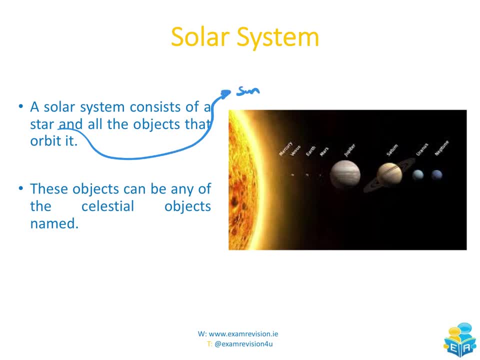 as well as all of the objects that orbit it. Now, these objects that orbit the star, they can be any of the celestial objects which we've previously mentioned. So in our solar system we have the main star, which is the sun. we have all of the planets. 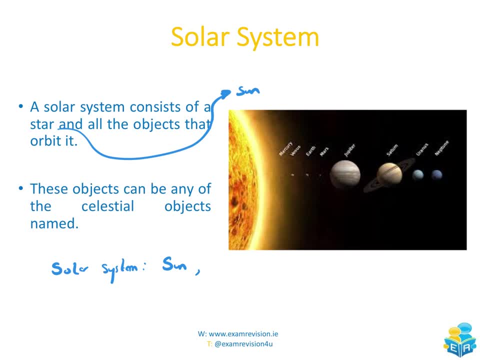 earth, mercury, venus, jupiter, neptune and so on. We have lots of moons, we have the moon. we have the sun, we have the moon, we have the moon, we have the moon. we have the planets. as I've mentioned, we can have dwarf planets in there as well. 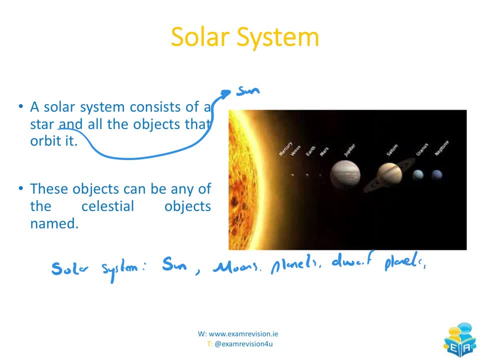 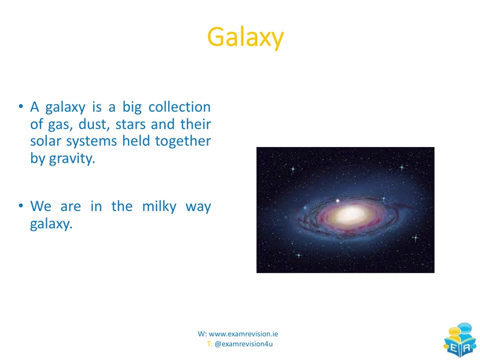 and we have millions and millions of asteroids, comets, meteors- all of those compose our solar system. Okay, so, it's the star and all of the objects that orbit around that star. A galaxy, then, is a big collection of gas, dust, stars and their solar systems, held together by 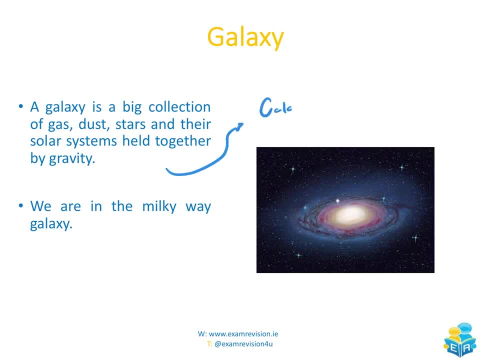 gravity. So, in essence, a galaxy is a combination of solar systems. Now, the galaxy that we're located in is the Milky Way galaxy. Okay, there is other galaxies out there as well, yet to be explored, but we can picture them. but the one that we're in is the Milky Way galaxy. 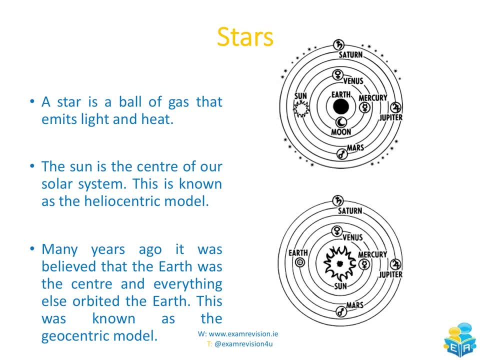 All right. so for the next couple of minutes we're going to focus in on all of the different celestial objects so we can differentiate them. So we're going to focus in on the Milky Way galaxy so we can differentiate between each one of those. Now, the main star in our solar system is the sun. 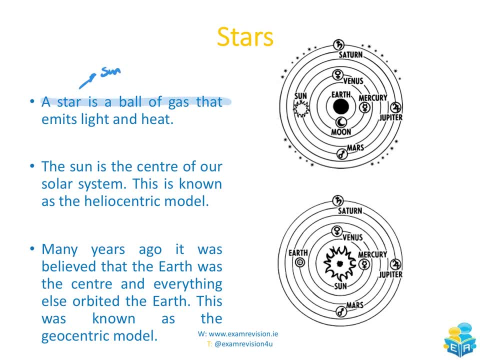 Now, by definition, a star is a ball of gas that emits light and heat. Okay, and we can see that from the sun. The sun is a big ball of gas. it does emit light and it does emit heat as well. Now, we know nowadays that the sun is the centre of the solar system and everything else orbits. 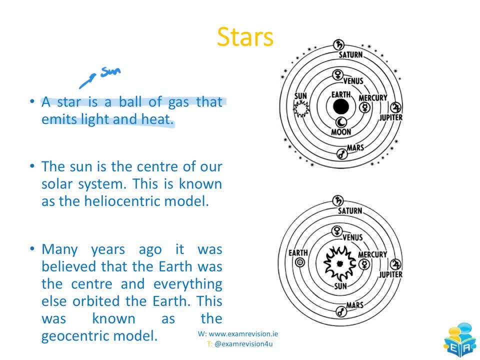 around it. So the idea of the sun being the centre of our solar system, that's known as the heliocentric model- Okay, but that hasn't always been the case. Many years ago, it was believed that the earth was the centre and that everything else orbited the earth. This was known as the geocentric model. Okay, so 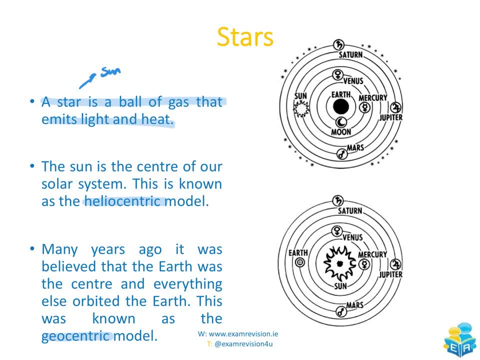 geo meaning land, land at the centre. So years and years ago, this model up here is what we believed it to be. Okay, the earth was at the centre. everything else, including the moon and the sun, orbited around the earth. But now, with advances in scientific discovery and better telescopes and so 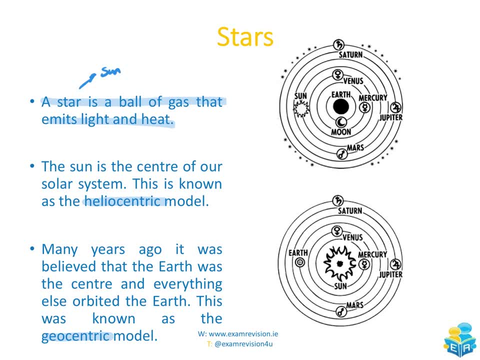 on. We know that the sun is the centre of the solar system. everything else orbits around that, including our cells. Okay, so us and all the other planets. we orbit around the sun. That's the heliocentric model. The geocentric one was the one with earth. Now that can be one example of a 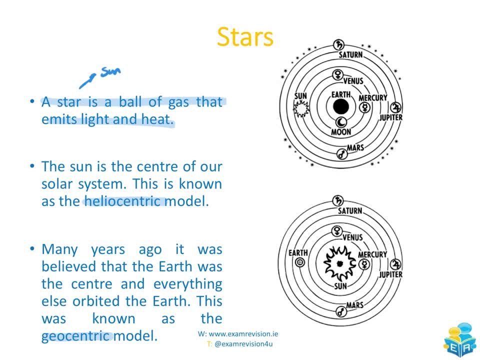 question which does appear in the final paper. The question normally comes up with outline one way in which our scientific understanding has evolved or changed over time. This is a perfect example to give for that. You could mention about how in the geocentric model. 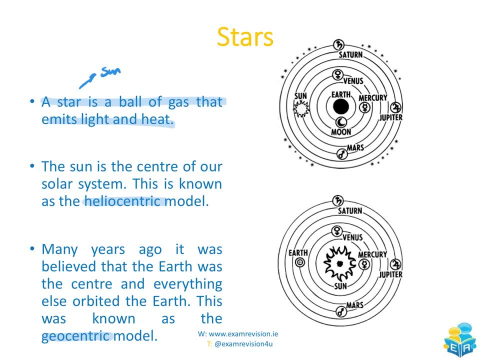 we used to believe that the earth was the centre of the universe. everything orbited around that. Now we know, in the heliocentric model it's not the case. the sun is the centre of the solar system. everything else revolves around that. okay, So that is an example you could use for that particular. 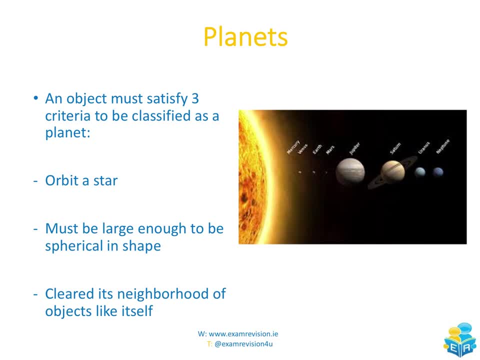 question. The planets, then, are the next thing We're going to focus in on. this is a very, very common exam question. So for something to be classified as a planet, that was obviously the famous case a couple of years ago where Pluto was declassified as a planet. 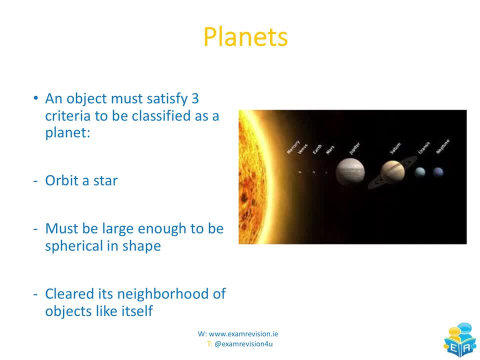 Then later classified as a dwarf planet, selected as a dwarf planet. before an object to be classified as a planet, as a planet, three criteria need to be satisfied: It must orbit a star. okay, The star we orbit is the sun. The planet must be large enough to be spherical or roughly spherical in shape. You're. 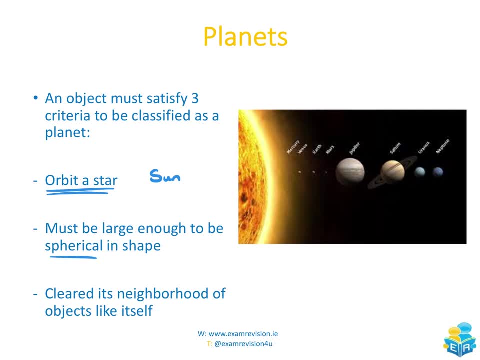 never going to have a perfect sphere, but it has to be large enough to be roughly spherical in shape, okay, And it also has to have cleared its neighborhood of objects like itself, okay. So it has to have a clear orbit. So, if all three of those criteria are satisfied, 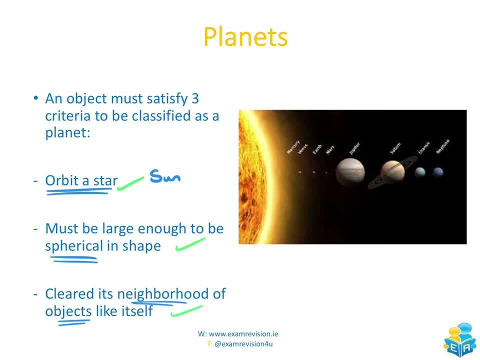 it's classified as a planet, Even if it misses out on one of them, it cannot be classified as a planet, So really important that all three are being met before an object is classified as a planet. So in our solar system then we have eight planets. We can see them here in the diagram. 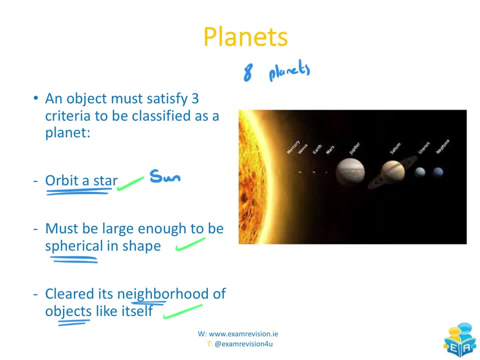 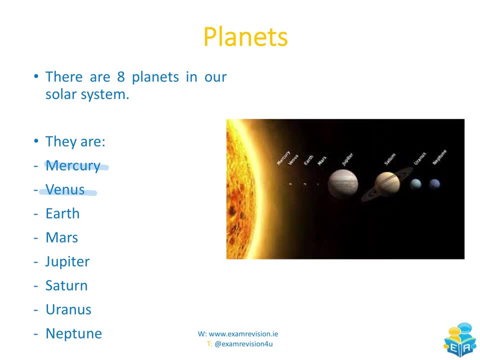 We have Mercury, Venus, Earth, Mars, Jupiter, Saturn, Uranus and Neptune. Now, I mentioned these planets on the last slide, so just to spell them out here we have Mercury, Venus, Earth, Mars, Jupiter, Saturn, Uranus and Neptune. Now it is important that we do know those. 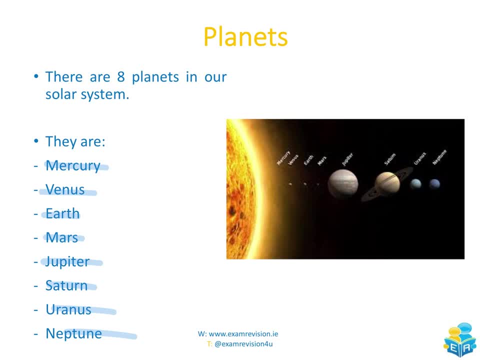 and they are actually listed there in order of closeness or proximity to the sun, the first one being Mercury, closest to the sun and then Neptune being furthest away. So if you want to remember which one is which, or a little device for remembering all of these, 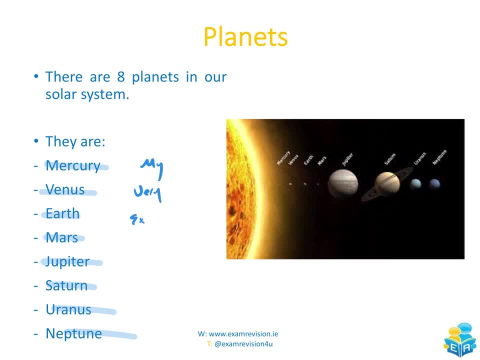 if you just remember, my very excited mother just served us nachos. Okay, because if you look at the first letter of each one of those, it links up to the first letter of the planet. Okay, so really important that you do know the eight names of the planets. 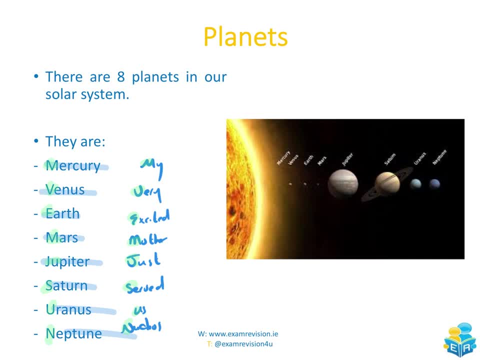 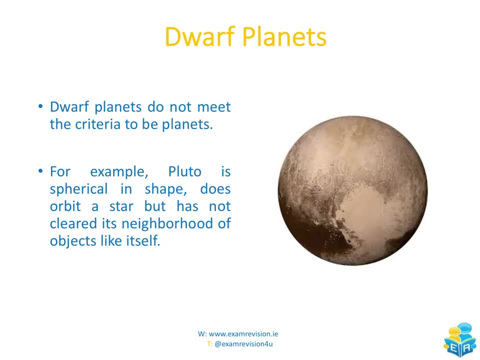 but do also know the order of them as well, because that can come up as a question: knowing which one is closest to the sun and which one is furthest away. Now, I mentioned already about the famous example there of Pluto being demoted as a planet. 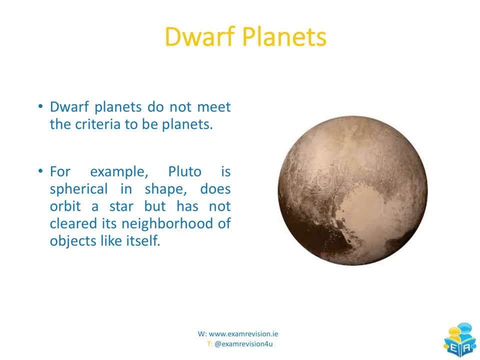 So dwarf planets do not meet the criteria to be planet. Okay, so think back to the three criteria. They don't meet all three. For example, Pluto is spherical in shape, so it meets that one. It does orbit a star, so it meets that one. 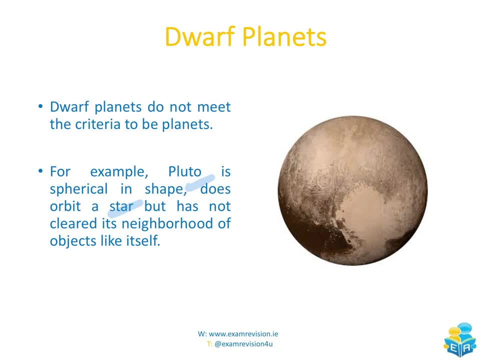 but it has not cleared its neighborhood of objects like itself. Okay, so it was declassified as a planet a couple of years ago and it is now referred to as a dwarf planet. So dwarf planets. they don't meet all of the criteria to be classified as planets. 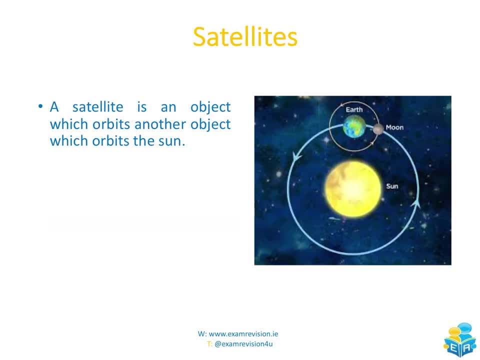 Pluto again being the famous example of that. Now, this is actually a good example of a planet. This is actually one of my favorite definitions which comes up in science. So we have the idea of a satellite. I'll come back to that in a second. 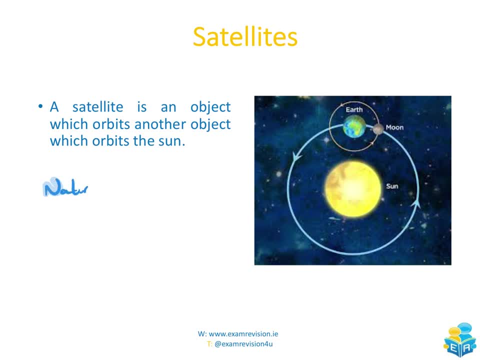 but we will eventually break the satellite down into natural satellites and artificial satellites. So, by definition, a satellite is an object which orbits another object, which orbits the sun. Now, how does that make sense? Well, the famous example of a satellite is our moon. 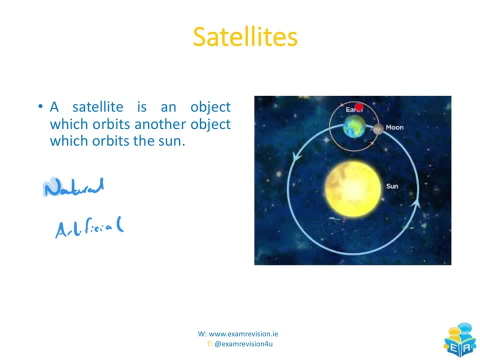 Okay, the moon is an object which orbits another object which in turn orbits the sun. Okay, so that's the definition there for a satellite: An object which orbits another object which orbits the sun. Okay, moon is an example of a natural satellite. 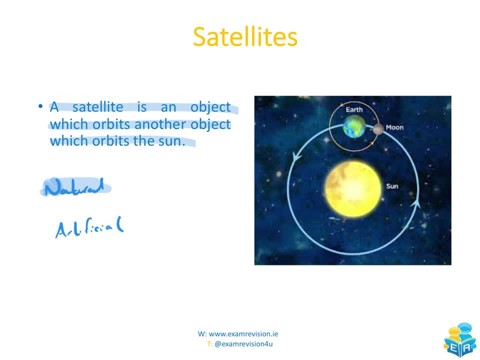 Okay, it's one of the celestial objects that happens to be a satellite, because they orbit another object which orbits the sun. We can have artificial satellites as well, So these are satellites which are intentionally sent into space. Okay, so the moon being an example of a natural satellite. 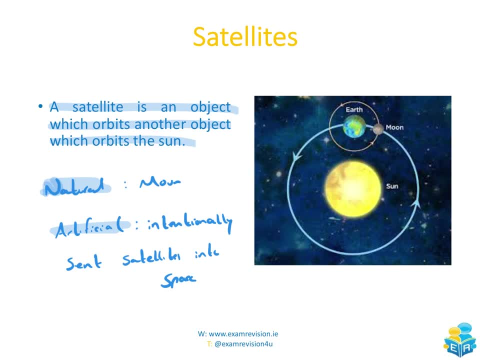 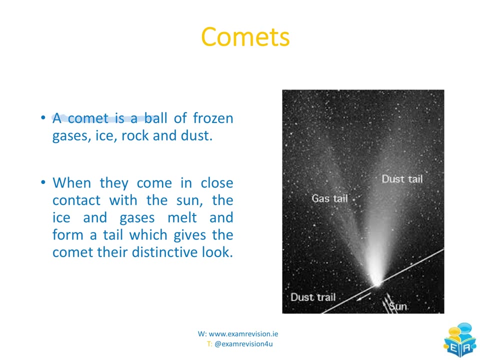 artificial satellites are ones which are intentionally put into space, But they too are technically classified as satellites because they will orbit another object which orbits the sun. Okay, so that's the satellites. Comets, then? A comet is a ball of frozen gases, ice, rock and dust composed of many of these. 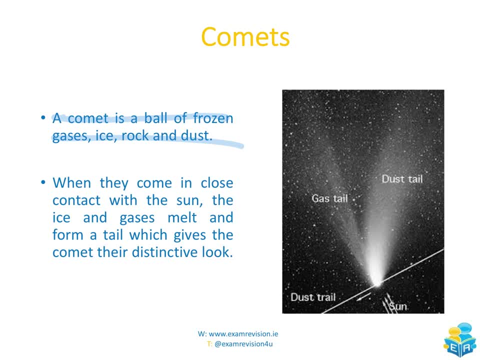 When they come in close contact with the sun, the ice and the gases are going to melt, given the temperature of the sun, And it's going to form a tail which gives the comet the distinctive look. Okay, so the tail is always formed behind the comet. 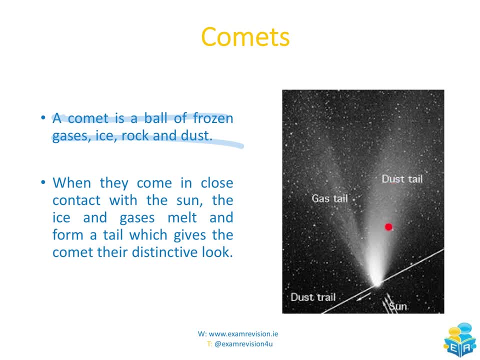 So if we have a look at this diagram over here on the right hand side, we can tell that the comet here is moving towards the sun, because there's the brightest point there, And we can actually see that the tail is forming behind it. Okay, the ice and the gases are melting and that's what's forming: the tail. 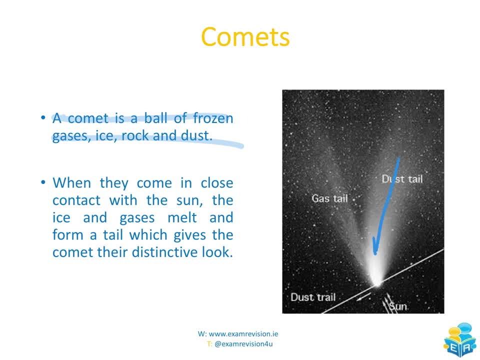 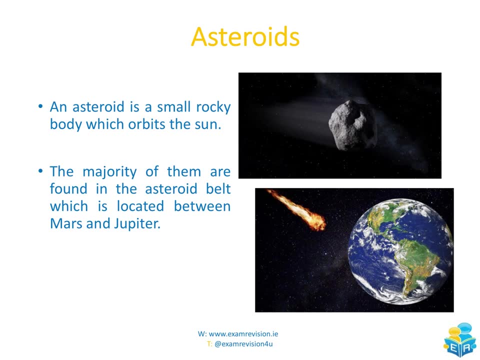 Okay, so if that's ever asked, we can say that the comet is moving in this direction here. So that's the asteroid belt. An asteroid, then, is a small rocky body which orbits the sun. Okay, so they're composed entirely of rock. 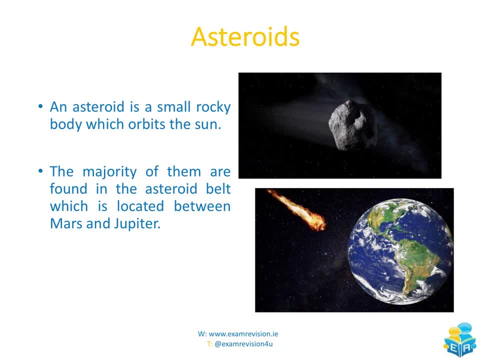 And the majority of them are found in the asteroid belt, and that's located between Mars and Jupiter. So many, many of these asteroids will be found there not really doing anything. They're just in orbit, But from time to time they can actually catch on fire. 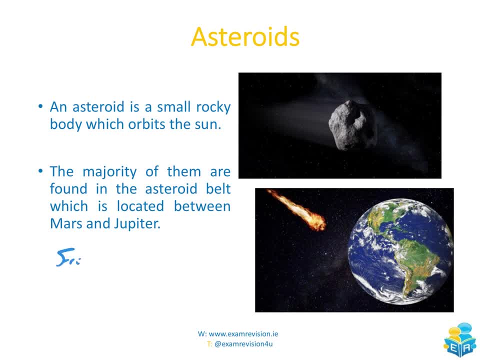 The reason for this is because, when they move, a frictional force is applied. Okay, and from time to time, if that frictional force, If that frictional force is really, really great, heat can be produced, and then it can start to burn. 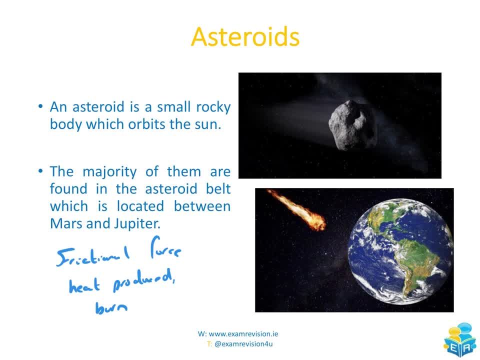 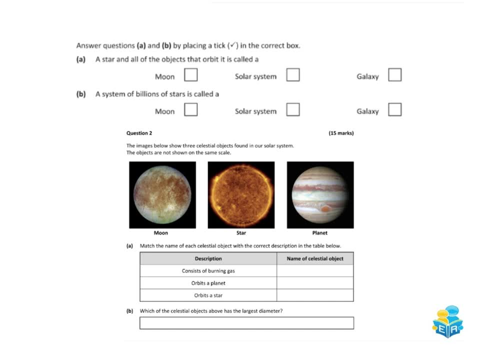 Okay, so from time to time that can happen, But just remember asteroids they're small rocky bodies composed of rock Majority, or majority of the time they're found in the asteroid belt. Okay so we're going to have a quick look at a question. 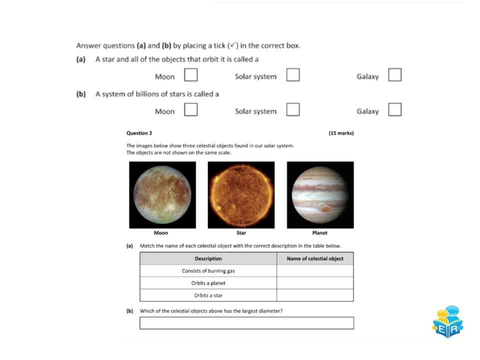 that's appeared in an exam before. based on all of this, It's actually two questions here. Answer questions A and B by placing a tick in the correct box. A star and all of the objects that originate from it. orbit, it is called. Is it A, a moon, a solar system or a galaxy? 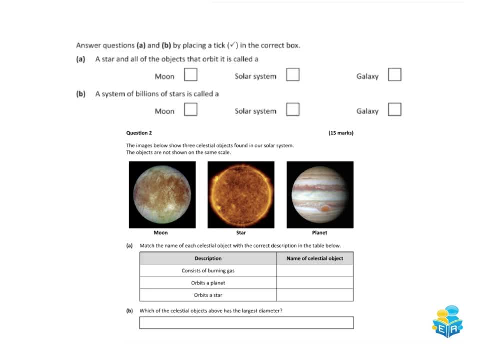 Well, it's not a moon, because a moon is a satellite, That's an object that orbits another object that orbits the sun. A galaxy is a collection of solar systems and lots of stars associated with that, And then the solar system is actually the required one here. 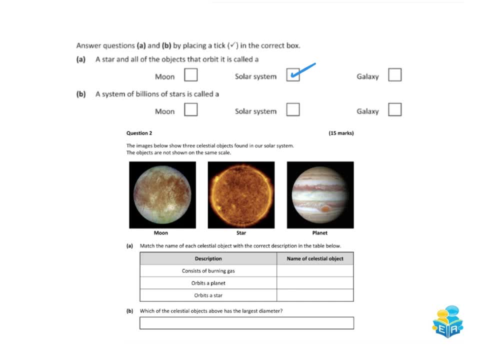 That's a star and all of the objects that orbit it, A system of billions of stars. Is it a moon, a solar system or a galaxy? This one here we mentioned a couple of minutes ago is the galaxy. Question two. The images below show three celestial objects. 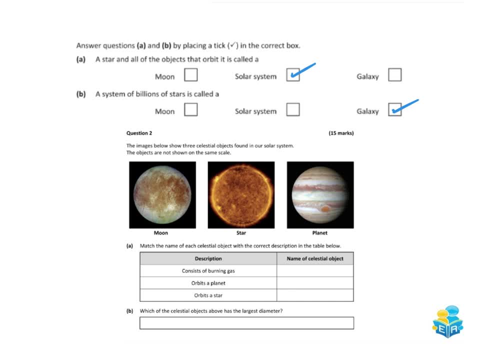 Which are found in our solar system. The objects are not shown on the same scale. So we have a moon, we have a star and we have a planet. Match the name of each celestial object with the correct description in the table below. 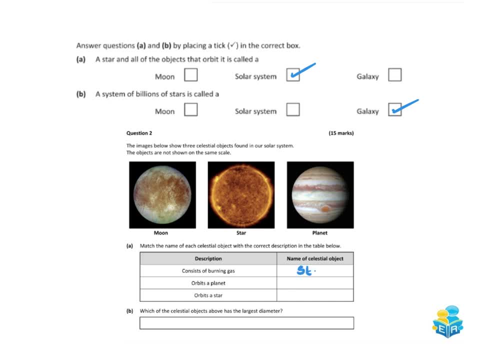 So it consists of burning gas- That would be the star, Orbits a planet That's going to be the moon. That's a satellite, And orbits a star, That's the planet. So our planet orbits the star, which is the sun. 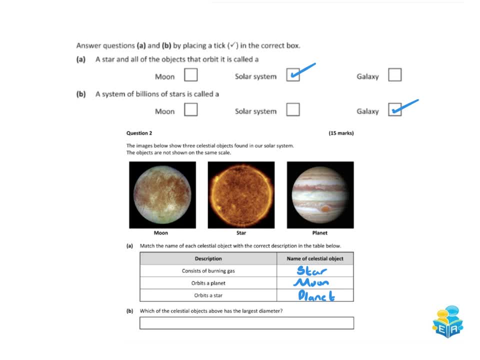 The moon orbits the planet, which in our case is Earth. Which of the celestial objects above has the largest diameter? This is going to be the star. It's the biggest one in our solar system. So that was all the celestial objects, And for the next couple of minutes we're going to focus in on the Earth. 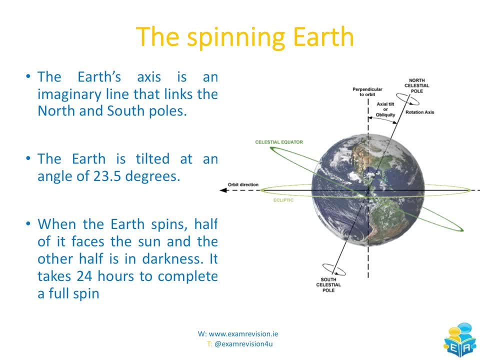 And more specifically, the Earth's tilt and how this is responsible for the seasons which occur on Earth. So the Earth's axis is an imaginary line that links the North Pole up here and the South Pole down here, So there isn't actually a physical line or a physical pole that goes through the whole of the Earth. 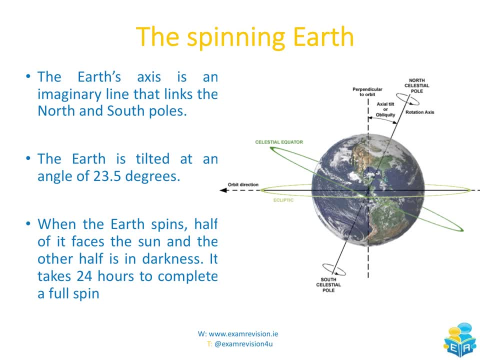 It's just an imaginary line Linking the North Pole and the South Pole. Now this tilt has been calculated to be at an angle of 23.5 degrees. So if we were to calculate this angle in here, it's 23.5 degrees. 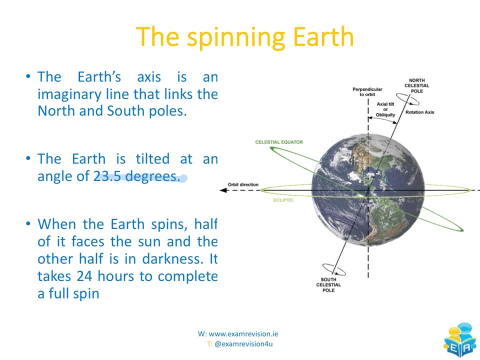 When the Earth spins, half of it is going to face the sun at all points and the other half is going to be in darkness. It's not receiving light from the sun. It takes 24 hours to complete a full spin, So for some of the day- obviously during summer we have longer days because we're tilted more- 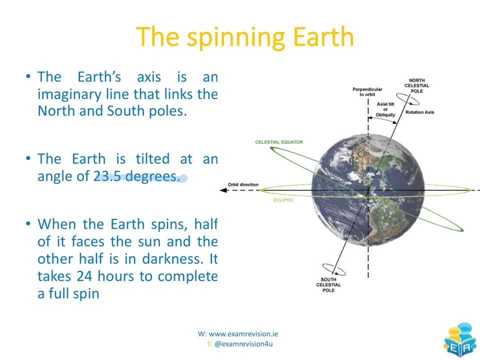 We're tilted more towards the sun, which we'll come to in a couple of minutes. In winter, we're tilted more away from the sun, So it's never really going to be a full 12 hours sunlight and daylight. It is going to change because of the tilt. 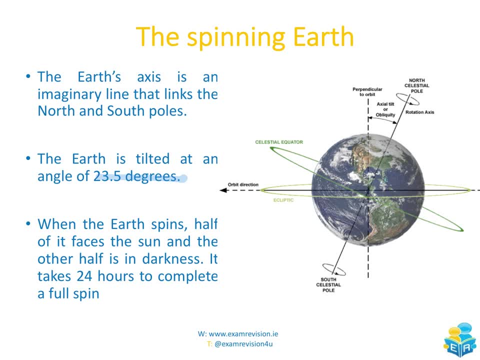 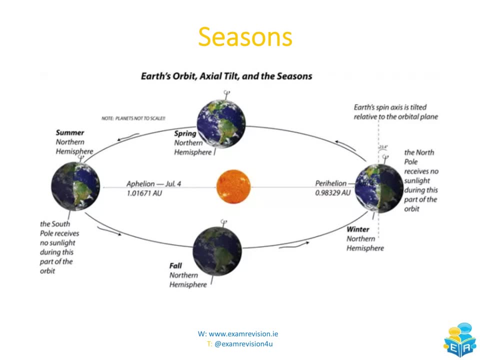 But half of it is going to face the sun, The other half is going to be in darkness. So this is a depiction of the Earth's seasons, So the Earth's orbit, its axial tilt and the seasons. So right here in the centre, we have our sun. 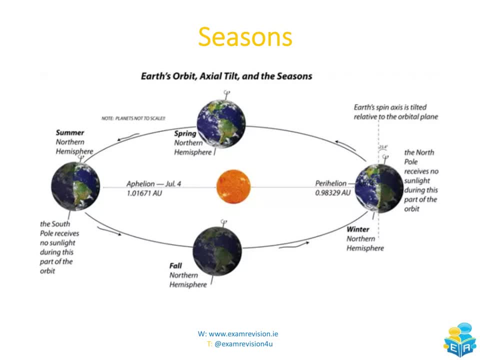 And we can see that in each one of the diagrams we have the same tilt. It's roughly 23.5 degrees. So the first thing we're going to have a look at over here is the idea of summer in the Northern Hemisphere, which is where we exist. 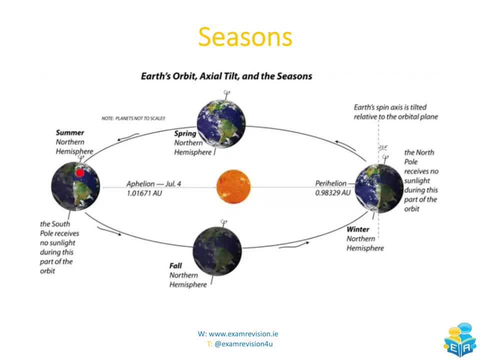 So in summer in the Northern Hemisphere, we can see here we're tilted toward the sun, We're in the Northern Hemisphere, we're tilted toward the sun. So this is why we have really nice long days, We have nice weather. But in the Southern Hemisphere this is when it is winter for them, because they're tilted away from the sun. 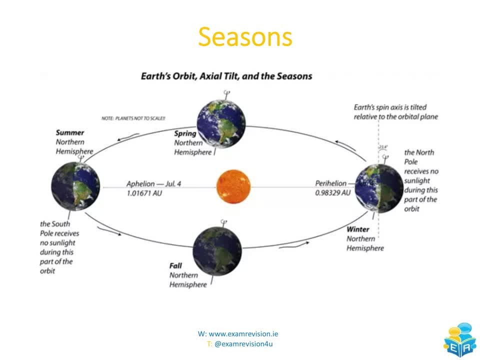 So they're not receiving as much sunlight. Days are shorter. Weather isn't as good. Now over here, when we're tilted away from the sun in winter, It's winter in the Northern Hemisphere. We're not receiving sunlight. The weather is a little bit poorer. 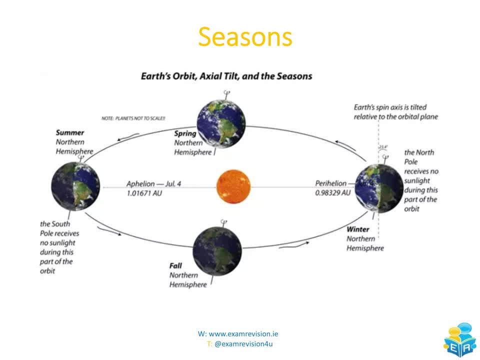 It's a little bit colder, But the Southern Hemisphere is getting really nice weather. It's summer in the Southern Hemisphere, So that's why, when we're celebrating Christmas over here, If you know anybody that might be in Australia, for example, They might actually celebrate Christmas Day on the beach because the weather is so good down there. 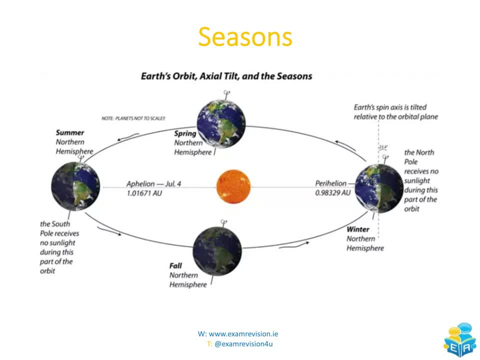 They're in the Southern Hemisphere, They're tilted toward the sun. We're tilted away from the sun, Okay, and then spring and autumn are kind of in between, So between summer and winter we're beginning to tilt away, So the days are getting a little bit shorter. 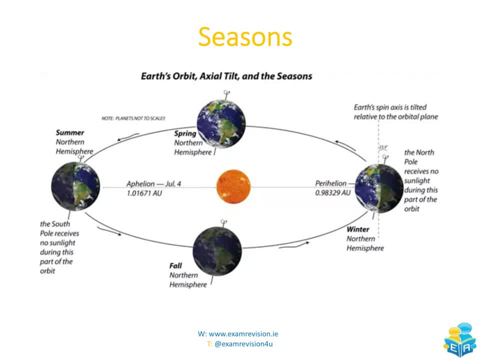 The weather is getting a little bit poorer Until we get into winter time, when we are not receiving sunlight. Opposite happens then in spring. So we're beginning to get to a point where we're tilting toward the sun. So the weather is getting a little bit better. 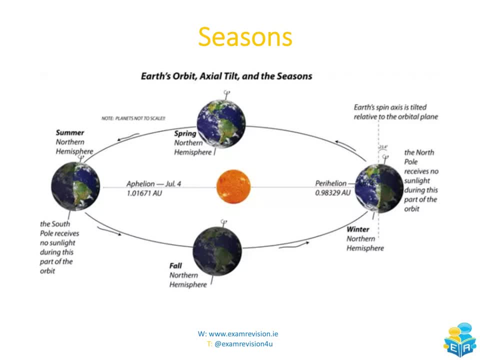 But in all of these cases we are tilted at 23.5 degrees. Okay, so at summer time we have longer days, We're tilted toward the sun. Winter time we're tilted away from the sun. So that's the seasons. So when we actually mention a season, it's just a division of a year. 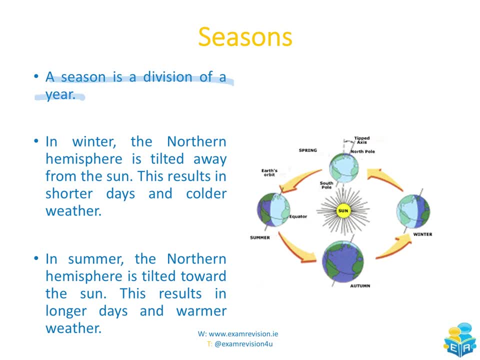 Okay, so if we divide it into four seasons, So we have summer, autumn, winter and spring, Okay, Therefore, three month divisions of the year. In winter, Okay, so say November, December, January time for us. The northern hemisphere is tilted away from the sun. 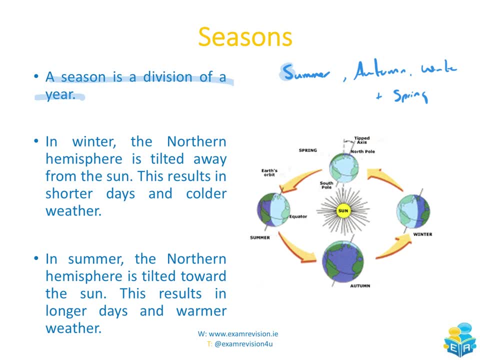 This results in shorter days and colder weather. But in summer the northern hemisphere is tilted toward the sun. This results in longer days and warmer weather. The southern hemisphere is the direct opposite of that. We've went through this already. We just have a quick look at it again. 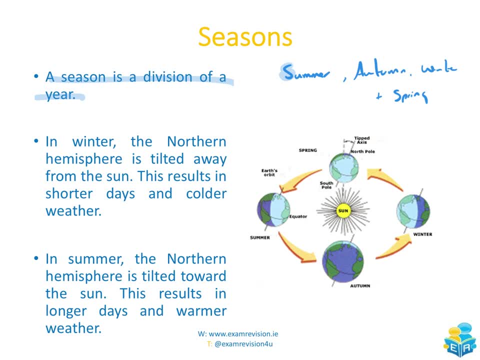 So there's summer time. We're in the northern hemisphere, We're tilted toward the sun, So we're going to get longer days, better weather. The southern hemisphere is not going to receive that For our winter. The northern hemisphere is tilted away from the sun. 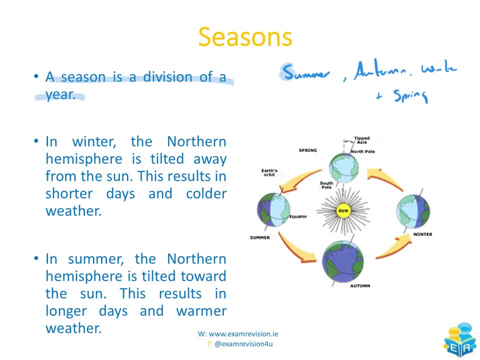 So we have shorter days, colder weather. The southern hemisphere is actually going to get the better weather here And then in spring. That's when we're beginning to tilt toward the sun. So we're starting to get nicer weather. In autumn we're starting to tilt away from the sun. 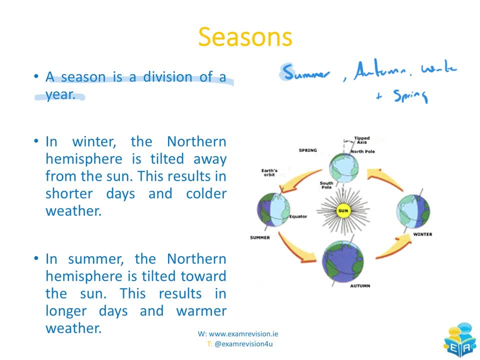 So that's when the poorer weather will begin to start. Okay, So that's the seasons. It's just a division of the year. We've summer, autumn, winter and spring, And it's because of our tilt. Are we tilted toward the sun, for longer days and better weather? 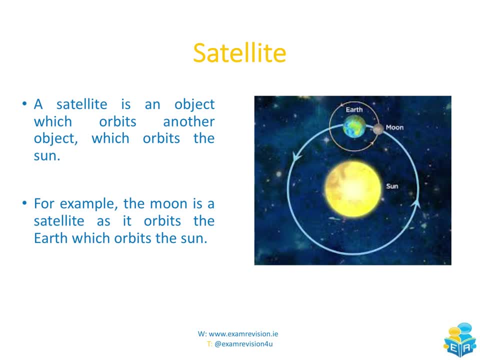 Or tilted away from the sun. So we're going to be focusing on the moon now for the next couple of minutes And the phases of the moon. Okay, So why does the moon look different when we look it up to the sky at night? 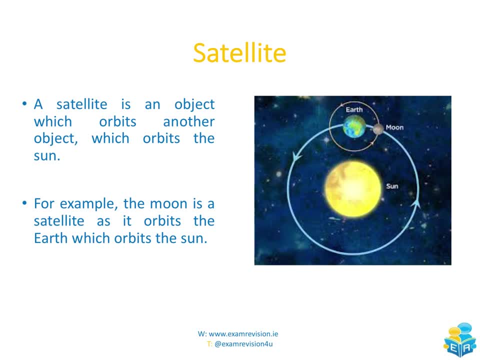 So, just before we move on to that, Just to come back to the definition: A satellite, It's an example. A moon is an example of a satellite, It's a natural satellite. A satellite is an object which orbits another object, which orbits the sun. 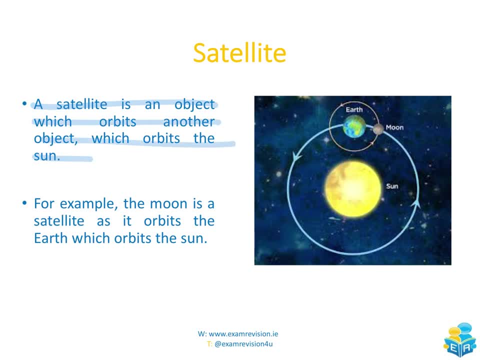 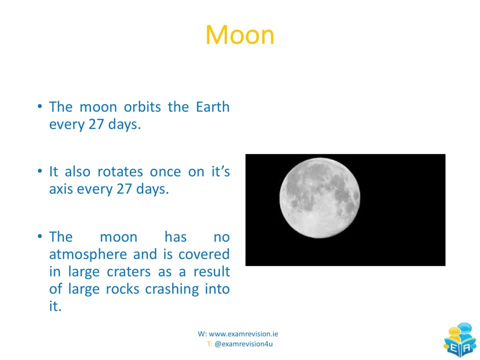 So the moon is an example in this case Because it orbits the earth. The earth orbits the sun. So it comes back to the definition An object which orbits another object which orbits the sun. Now the moon orbits the earth every 27 days. 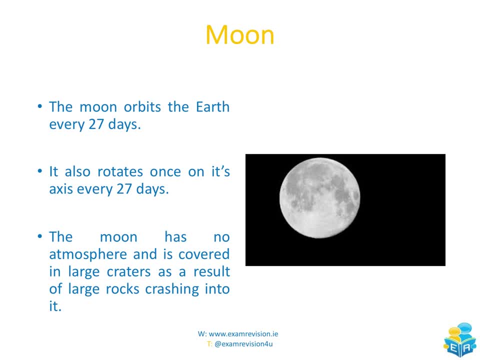 Okay, So once every 27 days it'll be back in the same position it started, But it also rotates once on its own imaginary axis every 27 days as well. So not only do we have our earth here, We have our moon out here. 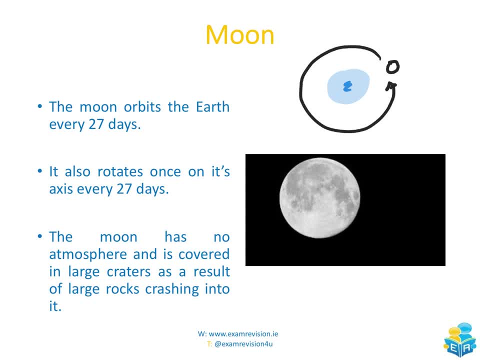 So once every 27 days, The moon is going to return to the same position, But at the same time, On an imaginary axis, The moon is also spinning, Okay, So it rotates once on its axis every 27 days. So that's a really important note to mention there. 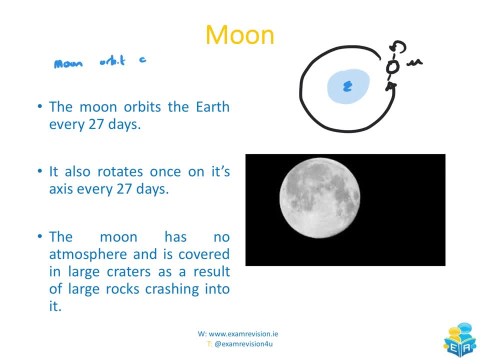 The moon's orbit And axis rotation Are approximately the same length. Okay, And it's because of this, I'll write this down here. Okay, So it's because of that That we only ever see one side of the moon. 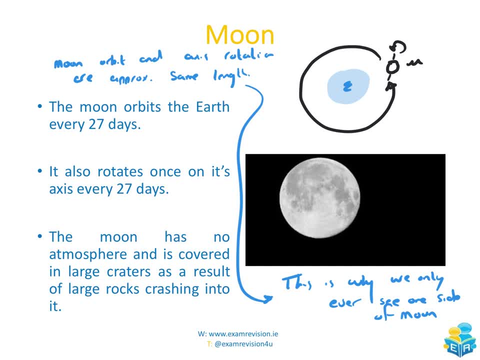 It's because the moon orbits the earth every 27 days, But it's also rotating on its axis every 27 days, So because they're approximately the same. That's why we only ever see one side of the moon, And you might have heard the other side referred to. 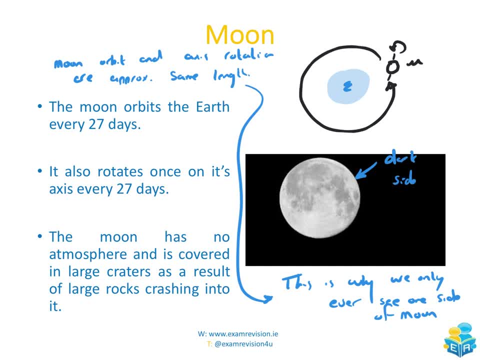 As the dark side of the moon. That's the side of the moon that we don't actually see Now, important to note here as well. The moon also has no atmosphere And is covered in large craters. This is as a result of large rocks crashing into it. 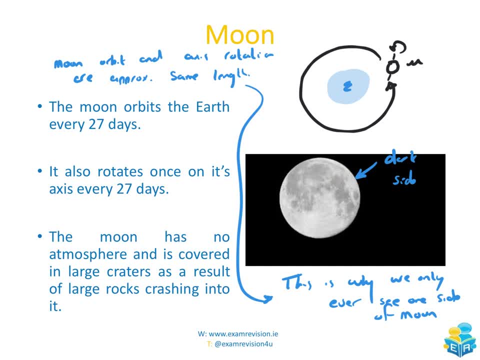 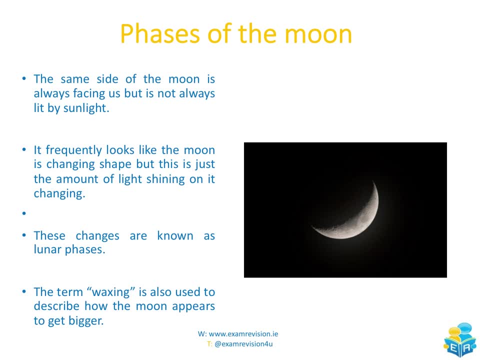 And you can see some of those craters in the diagram over here. Okay, So that's the moon. Now, we've mentioned this already About how we're always seeing the same side of the same face of the moon, But we're not actually seeing it all at the same time. 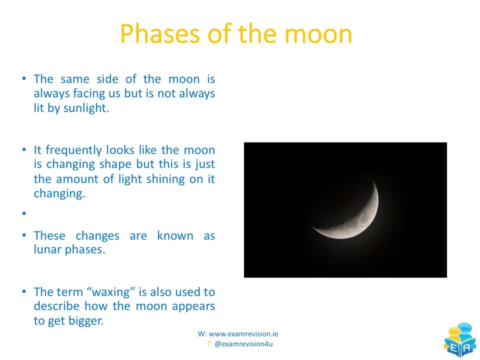 Okay, There's a period of the month where we'll see it all. Other than that, We're not going to see it all, And we'll only see little segments of it at a time, So the same side of the moon is always facing us. 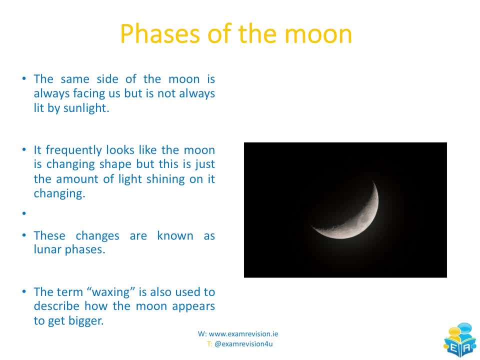 But it is not always lit by sunlight. So really important to mention here as well That the moon is known as a non-luminous object And the reason for that Is because it does not emit light. So yes, we can see it. 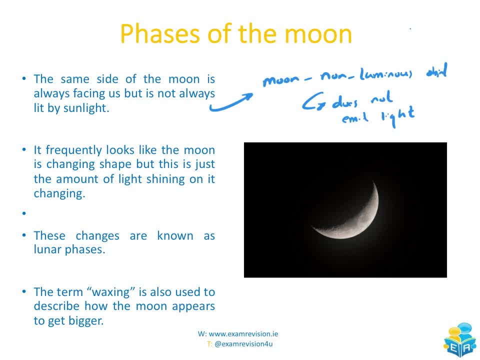 It looks bright from time to time, But that's the light of the sun. The moon itself is not actually emitting any light there, So it frequently looks like the moon is changing shape, But this is just the amount of light shining on it changing. 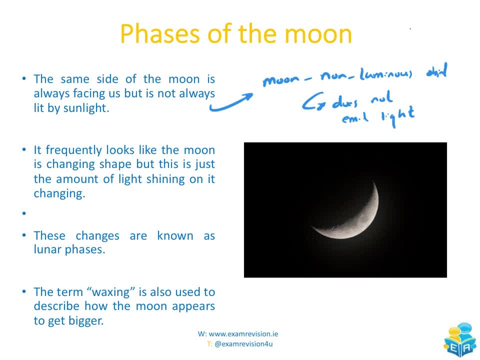 So if you can see the full moon, That's because the entire thing is being lit up by the sunlight. In this example over here, It's only the segment over here That the sunlight is falling onto And that changes from night to night. 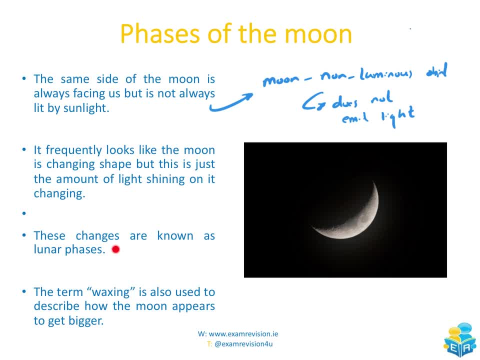 So these changes With the amount of light that's falling on it Is known as the lunar phases, Now the term waxing. We have two terms that we need to know here. We have waxing And we have waning. So if you were to go out to the sky tonight, 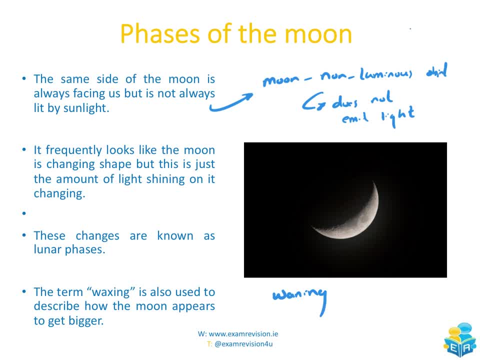 And look at the moon, Then go back tomorrow night, Then go back the next night, And go back the next night again If it appears that from night to night The moon is getting bigger Or you can see more of the moon. 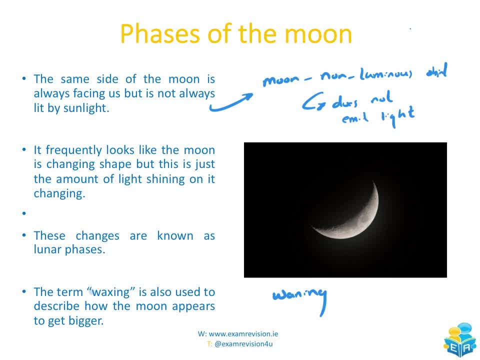 Or more of the moon is lit up by the sunlight. That term there is waxing, Okay. It's getting brighter, Okay. Waning, on the other hand, Is where it appears to get smaller. And just one more thing to note. 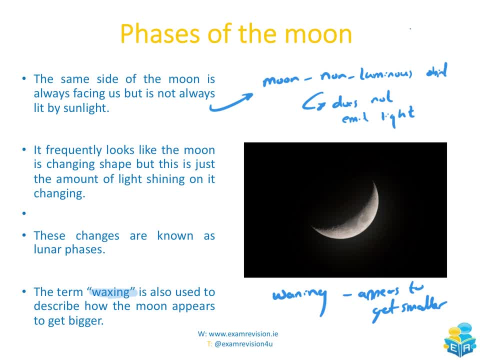 On this as well. It will always start from the right hand side of the moon. So if you couldn't see any of the moon at all, If it was in total darkness, It's from this right hand side That it will start. 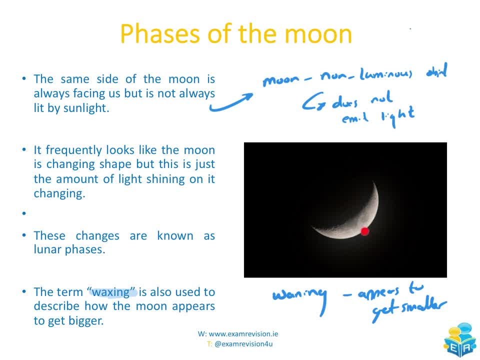 So at the minute, This moon here Is in the waxing phase, Because every night It's going to get bigger And bigger And bigger Until we can eventually see the full moon. Then, from the right hand side again, It's actually going to start to get darker. 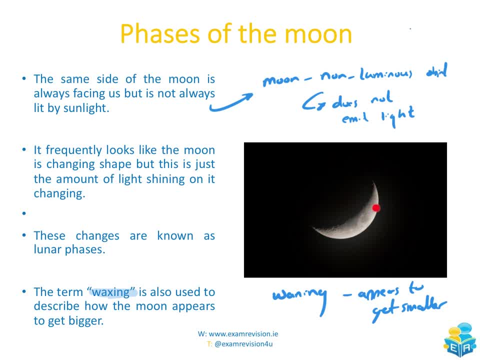 So it will start to get darker And darker And darker Until the full thing is in darkness, And then it will start to get brighter again. So just remember that for now, And I'll see you in the next video. Bye. 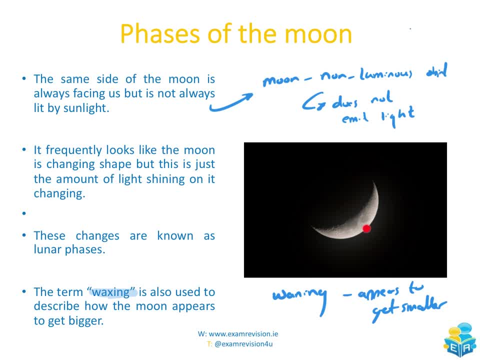 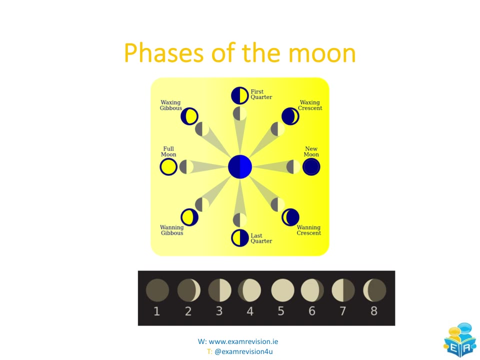 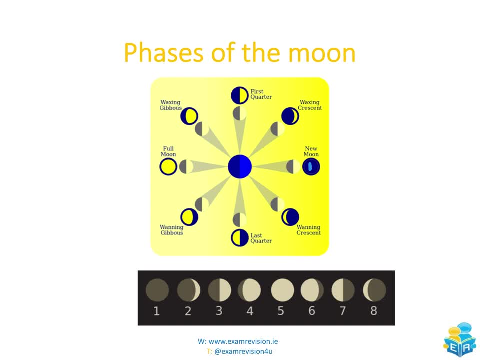 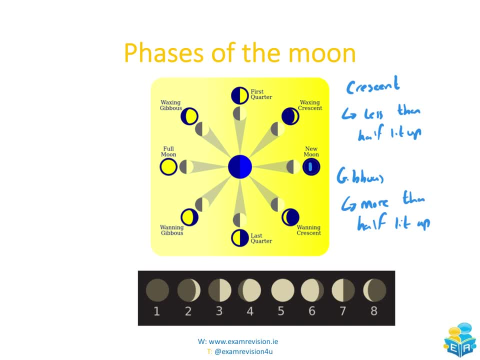 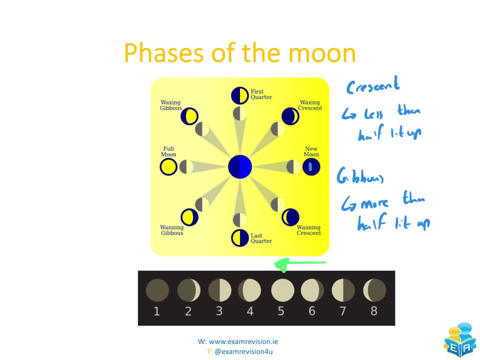 so it's going to start to get brighter from the right hand side. so stage two is the waxing crescent. okay, why is it called waxing and why is it called crescent? well, it's firstly called waxing because it's appearing to get brighter. as it goes from one to two, it's starting to get a little bit brighter. 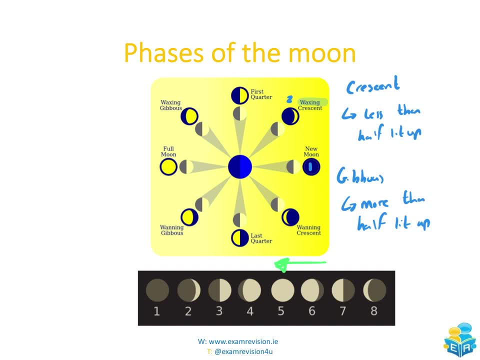 but it's also called a waxing crescent because less than half of it is lit up. if you have exactly half of it lit up, that's known as the first quarter. follow on from that, it's going to get a little bit brighter again. it's still appearing to get. 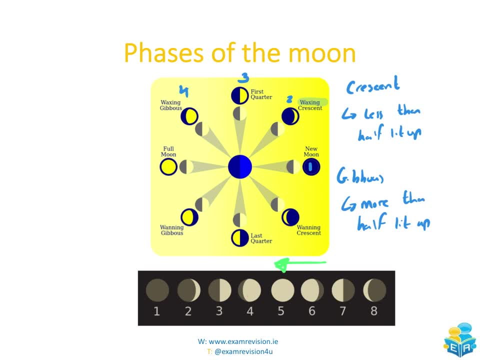 brighter night on night. it's getting brighter as we go from two to three, brighter as we go from three to four. so it's going to be called a waxing moon, but because more than half of it is now lit up, it's a waxing gibbous moon. okay, so we're combining waxing and waning with gibbous and. 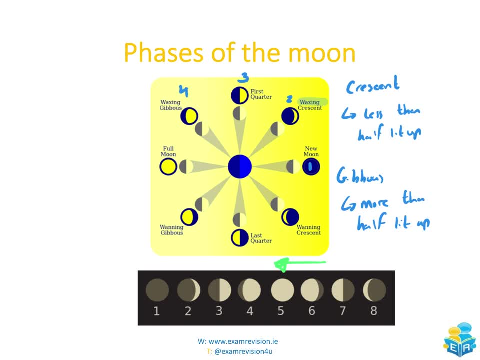 crescent. okay, we get to the waning one in a minute stage five. then this is our new moon. this is when we can see the full thing. okay, i'll come back to that in a second six, once it's been fully lit up. it's going. 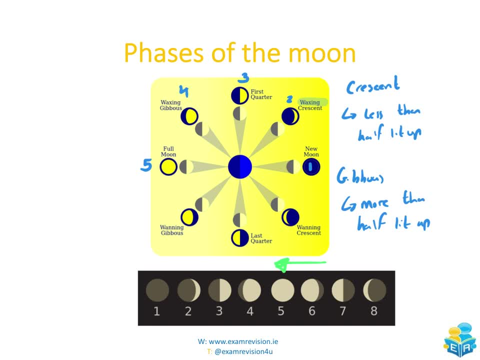 to start to appear to get darker. if it's starting to get darker, that's the waning moon. okay, it's getting darker from the right hand side. it's coming in from the right hand side again, but it's a waning gibbous because still more than half of it is lit up. we will have our last quarter. 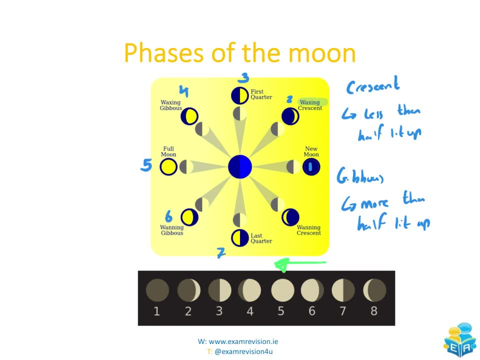 so that's number seven, and then number eight is going to be our waning crescent. so it's still getting darker in from the right hand side, but less than half of it is lit up now. so it's a waning crescent and then eventually all. 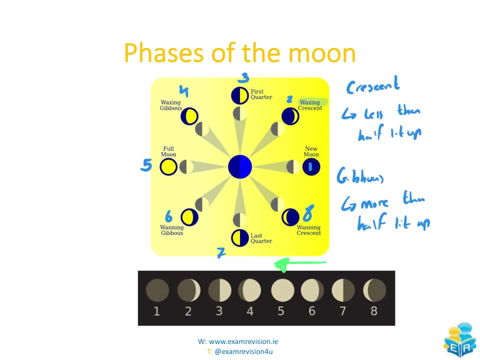 of it will be in darkness. so we will start off with our new moon again. now one thing to to keep in mind: generally we will have one full moon per month, per calendar month. that is okay. so say, once in january, once in february, once in march, if we get a second full moon in the same calendar month. 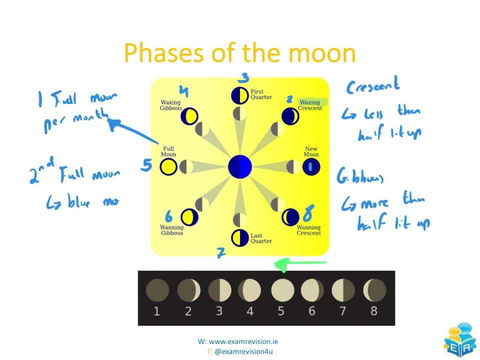 that's referred to as a blue moon. it doesn't actually mean that the moon is blue, it's just the term that's used for the second full moon in one calendar month. doesn't happen all that often, but it is important to know. so the terms you need to know here are waxing and waning, and then gibbous and crescent. okay, 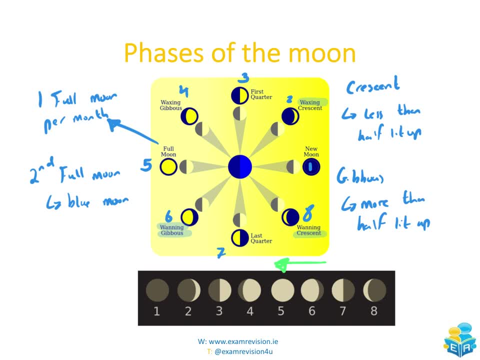 they're really important. so, waxing, waning, gibbous and crescent, they are all the phases of the moon, and it can come up as a question as well to be able to name the phase of the moon just by looking at one of these diagrams down here. so the first phase is in june, ok. then the next phase is in february, and then june is in june. effect one, phase two is coming. 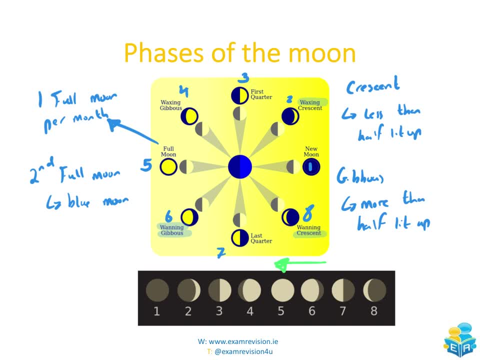 is the constitution of the moon, because june is a concept in june. so in the later presidential period june is ruled as a welche to motion of friday and所以 down here. so the first thing i would look at: is it more than half? is it less than half if it's more? 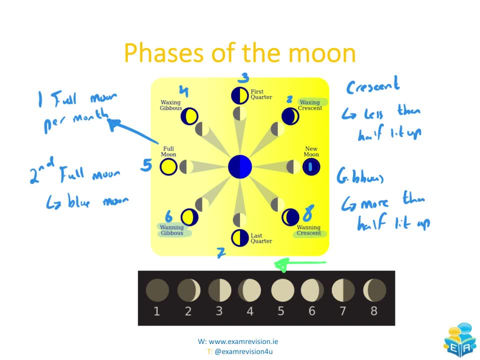 than half, it's gibbous. if it's less than half, it's crescent. is it getting brighter from the right hand side, or is it getting darker from the right hand side? if it's getting brighter, it's waxing. if it's getting darker, it's waning. okay, so we talked through this already, but we're just going to put 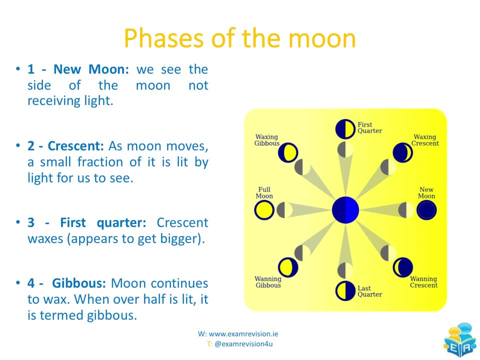 it down into text now. so, very first we have our new moon. so this is where none of the moon is receiving light. so we see the side of the moon not receiving light. it looks like it's in darkness here. okay, that was number one. following on from that, we have our waxing crescent. so, as the moon, 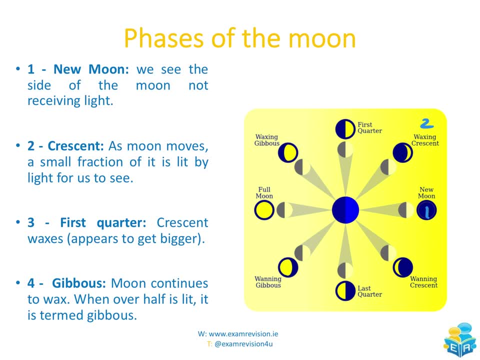 moves. a small fraction of it is lit up by light for us to see, so we can only see a small little bit of it. it's a waxing crescent. we then have our first quarter, so this is where it still gets bigger. the crescent waxes, it appears to get bigger and it looks like half of the circle we can see is. 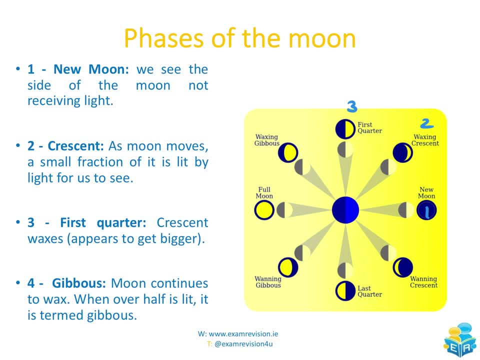 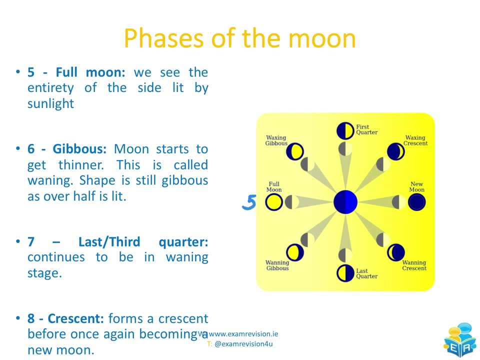 okay, that's the first first quarter. number four: this is our waxing gibbous, so it still appears to be getting brighter. more and more light is falling onto it. it's termed gibbous because more than half of it is lit up by light. number five is our full moon, so we see the entirety of the side lit. 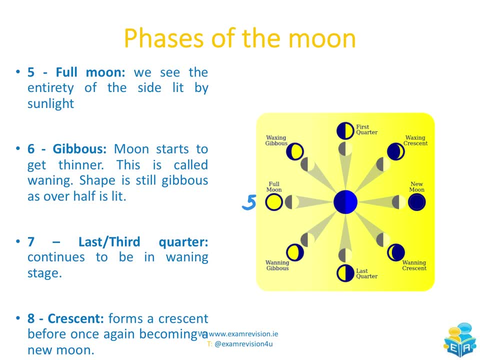 up by the sunlight. obviously, there's still a full side of the moon that we can't see. that's in darkness on the other side, but the side that we can see is fully lit up by light. we then have our waning gibbous, so it appears to be getting darker now. it appears to be getting smaller, but it's. 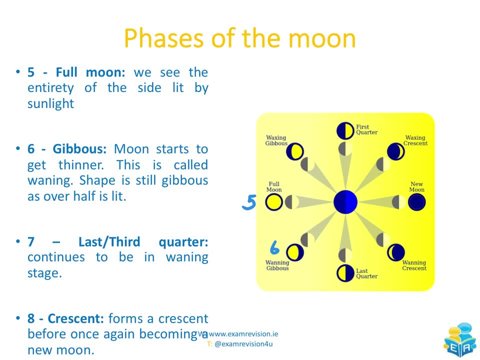 still more than half lit up, so it's a waning gibbous. we then have our last quarter, our third quarter. it continues to be in the waning phase and half the side that we can see is still lit up. the other half has now gone completely dark. we then have our waning crescent, so it still appears to 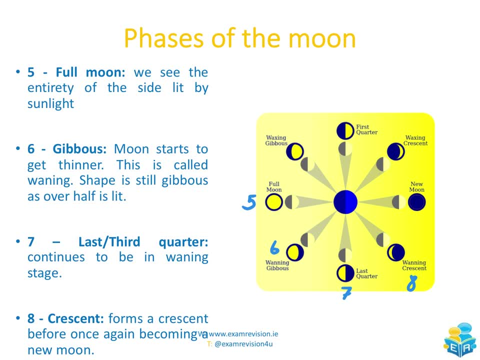 be getting darker. it still appears to be getting smaller. less than half of it is lit up in this case, so that's why it's referred to as a crescent. and then, eventually, we will go right back to the start here again, to our new moon, where it all appears to be in darkness, the side that we're seeing. 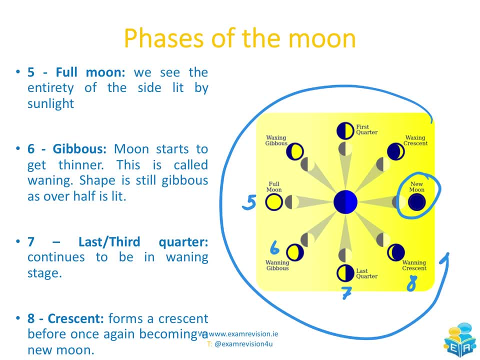 and the entire process then will start again. okay, so that generally happens. the same amount of time that the moon is going to rotate on its axes- between 27, 29 kind of days, so somewhere around that time frame it will go through the exact same phases again and again, and again, and just remember. 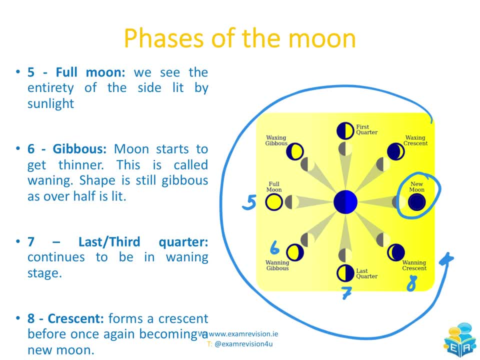 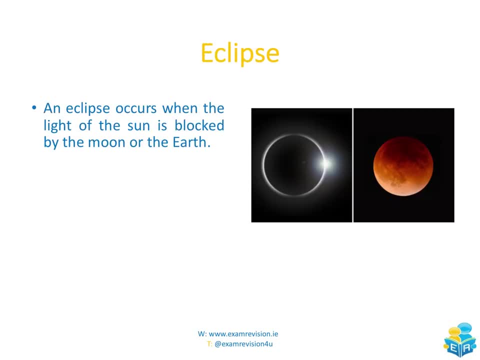 if you ever do have two of these full moons in one calendar calendar month. the second one is referred to as the blue moon. okay, so we're now going to combine the sun and the moon and the earth and we're going to start to have a look at eclipses. so there's two types of eclipses we can. 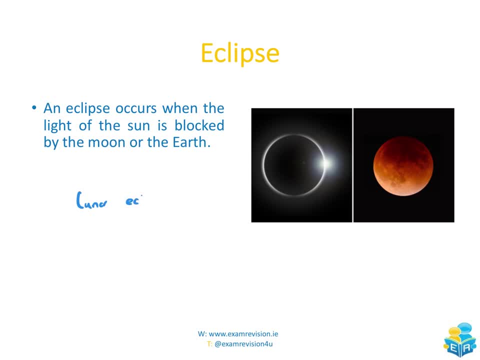 have lunar eclipses or we can have a solar eclipse. okay, so an eclipse occurs when the light of the sun is blocked by either the moon or blocked by the earth. if we have a solar eclipse, we're going to end up with this over here, so it's where the moon positions itself between the earth and the 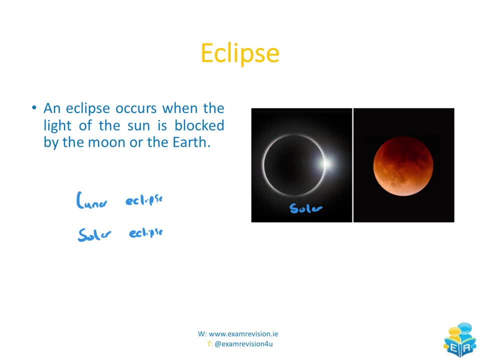 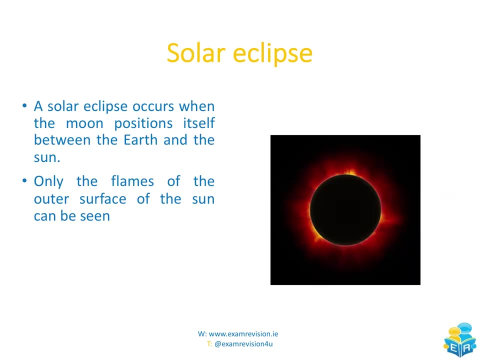 sun, and it looks like the sun is blocked off. we can only actually see the outside of it, a lunar eclipse. the earth's shadow is essentially falling onto the moon, so it appears more darker than it usually is, so that there would be the lunar eclipse. now we're going to focus first of all on the solar eclipse. we look at a diagram of how this. 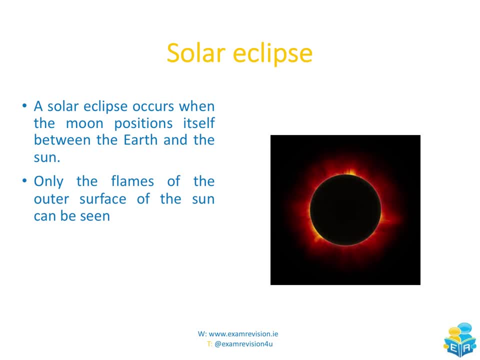 actually forms and then we move on to the lunar eclipse. so a solar eclipse occurs when the moon positions itself between the earth and the sun. so really roughly, here we have our sun, we have our earth over here, and the moon is going to position itself in here. okay, so the moon is. 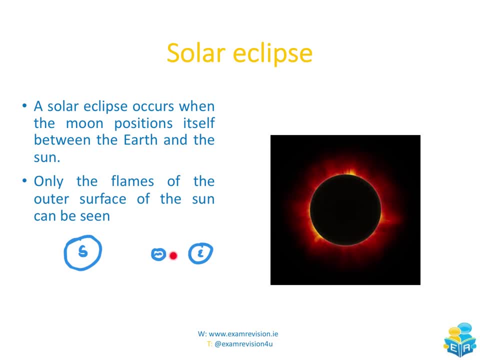 positioning itself in here, which means that if you are standing on earth, the moon is actually blocking it and appears that the full thing is covered. you can actually only see the flames on the outer surface. so that's the solar eclipse. we look at a more detailed diagram in a couple of 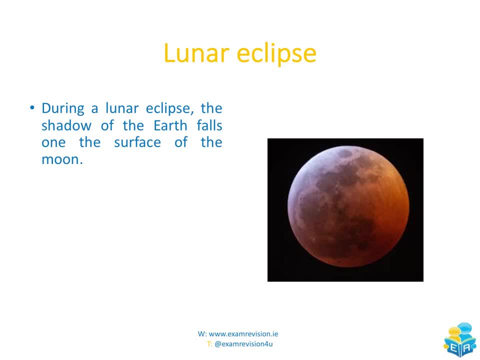 minutes, the lunar eclipse. on the other hand, then, during the lunar eclipse, this is where the shadow of the earth is going to fall on the surface of the moon. so we have our sun over here, we have our earth over here and we have our moon over here, so the sunlight that's trying to come from the sun. 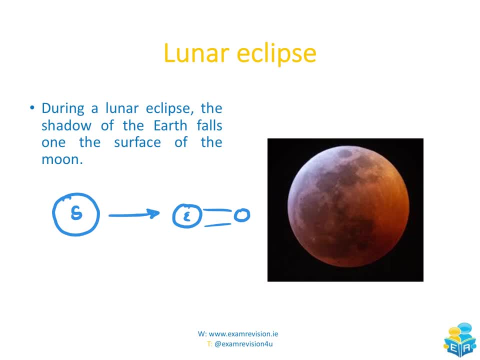 is going to be blocked by the earth and this is going to cast a shadow then onto the moon and it's going to appear like this over here. okay, so that's the lunar eclipse, and, again, we'll have a look at a proper diagram of this in the next minute or so. okay, we're going to start off with. 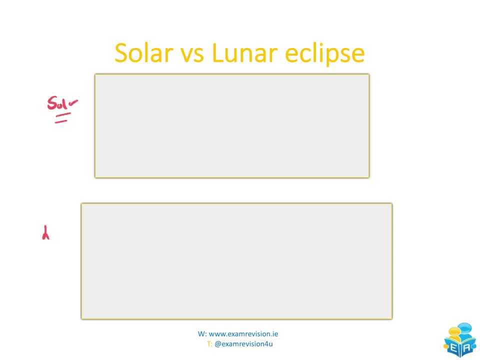 both of our eclipses here and look at diagrams associated with them. so we'll do the solar one first and then we'll move to the lunar one. so we have our sun, we have our earth and in between, we have our moon. okay, so if you were standing here on earth, what we should see is that the light from the sun is. 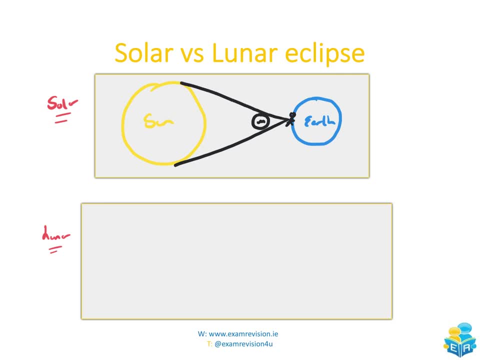 being blocked by the moon. okay, doesn't matter what direction this sunlight is trying to go, it's going to be blocked, so okay. so what's going to happen if you were standing here on earth? it's going to look like the sun is completely blocked off by the moon. you will only be able to see the outside flames. 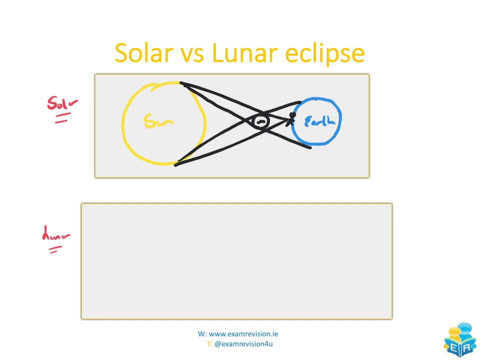 okay, we're going to form two different areas in here: this area in here which i'm about to do in green- normally i'll do it in gray, but just to make it stand out, that area there is called the umbra, which i will explain in a second- and this region out here, which i will do in red. 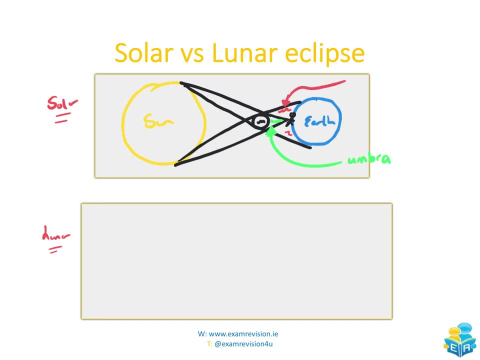 that's called the penumbra. so before i get to those, just imagine yourself. you're standing here. you can only see the outside of the sun. this is a solar eclipse because the moon has positioned itself here in the center and is blocking the sun. now, just to mention those two terms, umbra and penumbra. 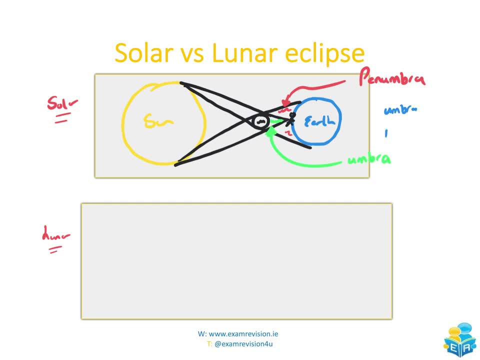 this is going to be the same for both types of eclipses: the umbra is the darkest shadow and this is the lighter shadow. okay, so that's just important to know. we would actually have our darker shadow in here. this would be the lighter shadow out here. okay, that's the solar eclipse. now for the lunar eclipse. 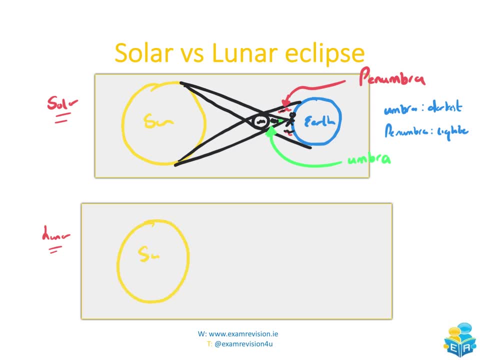 we still have the same object, so we still have our sun, our earth is going to be here in the center and we still have our moon, so it doesn't matter where the sunlight is trying to come from. it's going to be blocked off by the earth and shadows will start to form again and we're going to have the same object here in the 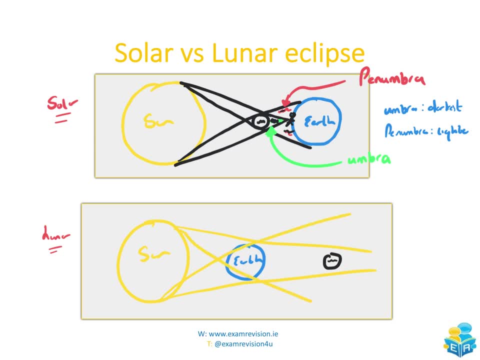 center again, which i get to now in a second. okay, so not the most perfect diagram, but you get the idea that will continue on. they'll eventually meet. so we have our two regions again. we've our umbra region and our penumbra region. this is going. 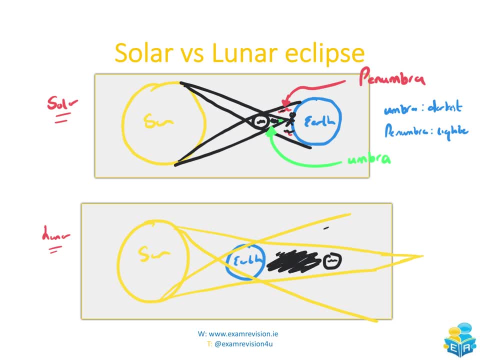 to be the darkest shadow in here. that's the umbra region. this is going to be a lighter region out here. okay, so that's our umbra region, then that's our penumbra region. so what's happening in this case? well, the light from the sun is going to be blocked by the earth. 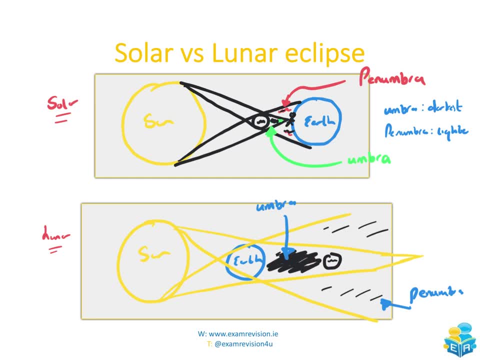 and a shadow is going to be passed on, passed onto the surface of the moon, so it's going to appear that the moon is in darkness. we'll still be able to see the outline of it, it's just going to appear slightly darker than it normally would. okay, there's a shadow after being cast onto the moon. 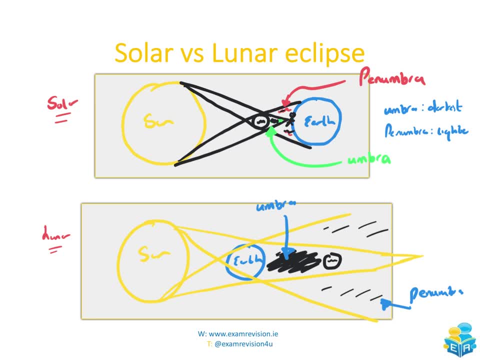 so that's the difference there between the solar eclipse and the lunar eclipse. it is really, really important to know those diagrams. i will show you proper diagrams that i didn't draw on the next slide, but it will be the exact same diagram. i will show you the proper diagrams that i didn't draw on the next slide, but it will be the exact. 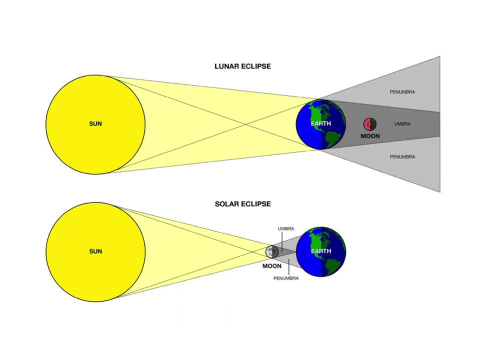 same idea. really important that you know those. so here it is again. there's the solar eclipse, which is the first one we looked at the sun on the earth. the moon is going to position itself in between and if you were standing here on earth, the moon is actually going to block the light coming down. 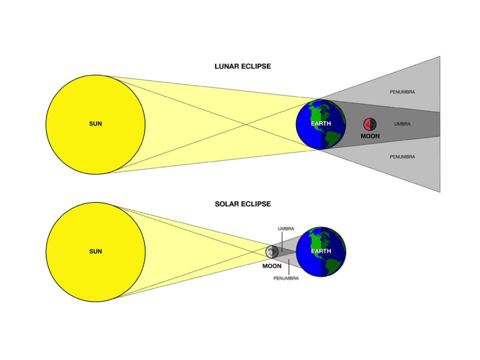 so it's going to appear that you can only see the outside of the sun. the rest of the sun is going to appear like it's covered by the moon for the lunar eclipse up here. the moon is going to position itself behind the earth. the sunlight that's coming from the sun. it's going to be blocked by the earth. 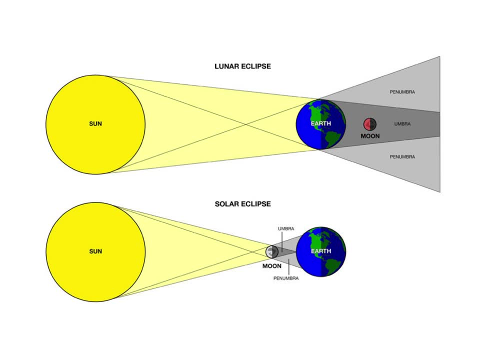 and then a shadow is going to be passed down onto the moon. okay, you'll still be able to see it. it's going to appear slightly darker, okay, and the two regions we have: our umbra region and our penumbra region. the umbra region is the darkest portion of the shadow. the penumbra region is the lighter. 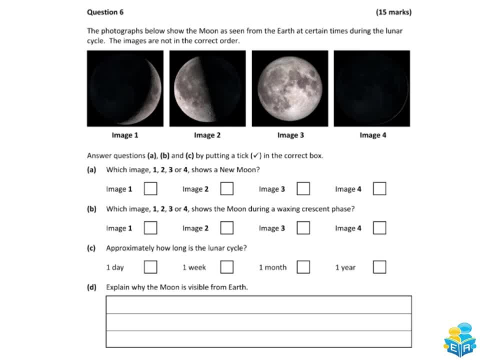 portion of the shadow. okay, so just to finish up, we're going to look at a couple of exam questions based on the entire content which we looked at today. so the photographs below show the moon as seen from the earth at certain times during the lunar cycle. the images are not in the correct 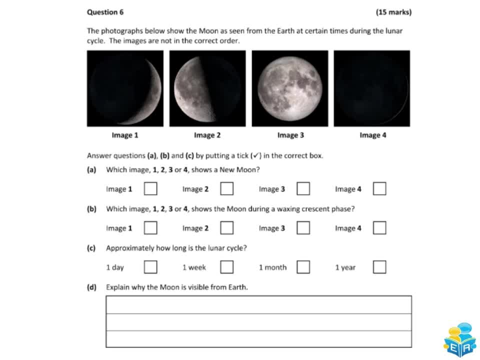 order. answer questions a, b and c by putting a tick in the correct box, so which image- one, two, three or four- shows a new moon? so a new moon is one of the two regions of the earth and the other is one of the other regions of the earth, and the other is where we can't see it. the full moon is where. 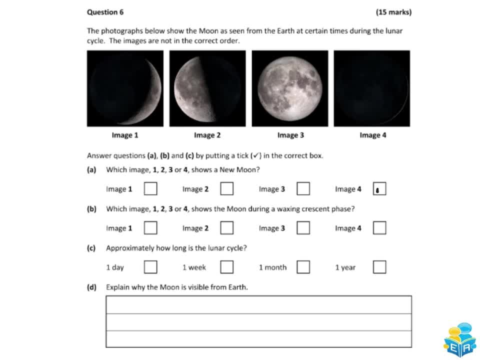 we can see it all. so the one here where we can't see it is image four, which image one, two, three or four- shows a moon during a waxing crescent phase. so crescent phase is where less than half of it is lit, so that would pinpoint towards this one here. a waxing phase is where it's getting brighter from. 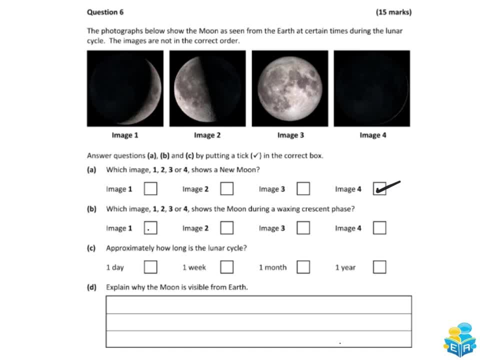 the right hand side. it actually meets that criteria there as well. so that's image one. approximately how long is the lunar cycle? that's roughly one month, okay, between 27, 29 days, so roughly one month, and explain why the moon is visible from the earth. so we can say here the 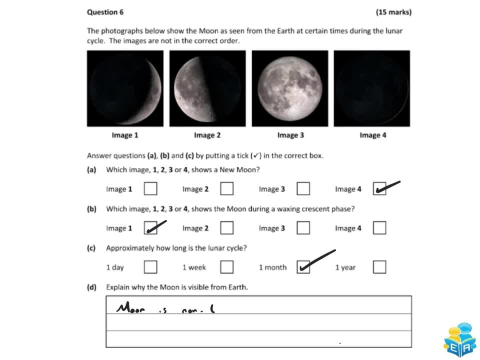 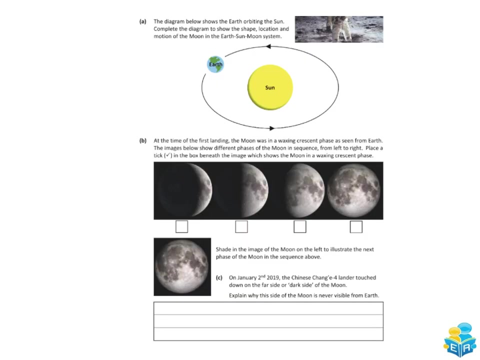 moon is non-luminous, it does not emit light, but we can see it because it reflects light from the sun, so it's not visible from the earth. okay, so that would have been the answer there for that. so this question here. the diagram below shows the earth orbiting the sun. complete the diagram to. 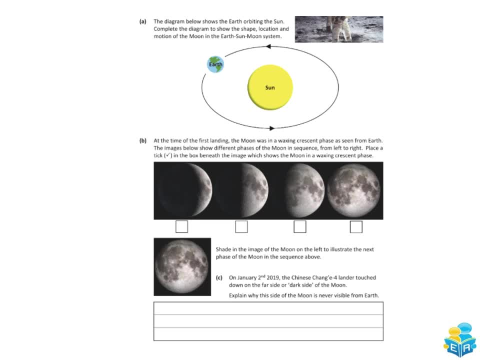 show the shape, location and motion of the moon. so the moon is going to be roughly here and it's also going to rotate or orbit around the earth. okay, so that's the moon. at the time of the first landing, the moon was in a waxing crescent phase, as seen from the earth. 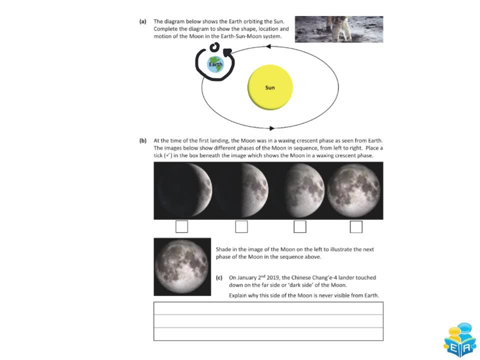 the images below showed different phases of the moon, in sequence from left to right. place a tick in the box beneath with the image which shows the moon, and the moon is visible from the earth in a waxing crescent face. so actually only one of them is in a crescent phase. this is um one of the. 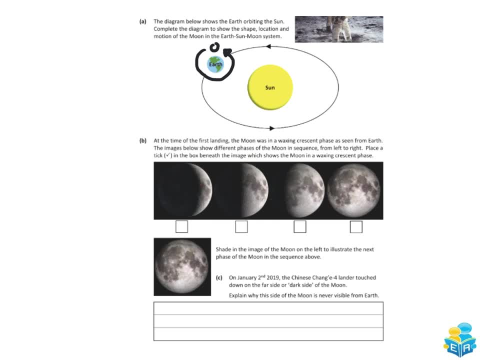 quarters. this is the gibbous moon. this is the full moon. this is the only one with a crescent. so that's this one here, shading the image of the moon on the left to illustrate the next phase of the moon in the sequence above. now remember when it starts to get lighter and when it starts to. 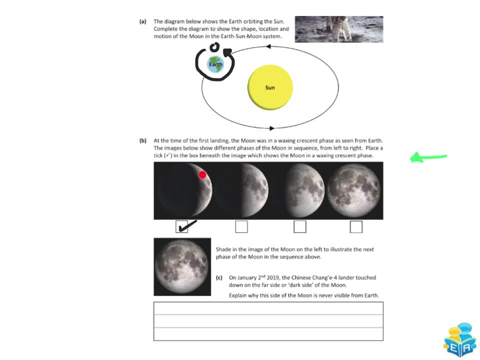 appear to get darker. it comes in from the right hand side. so here it was getting brighter from the right hand side, brighter from the right hand side, even more bright, even more bright. now it's going okay, but it's going to be, um, a waning, gibbous moon, so only this portion of it here is going to be. 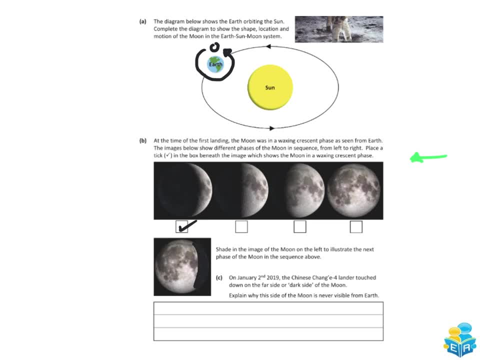 shaded off because more than half of it is going to be lit up. so on january 2nd 2019, the chinese changi four lander touched down on the far side of our dark side of the moon. explain why this side of the moon is never visible from the earth. so the moon rotates on its axis at the same rate. 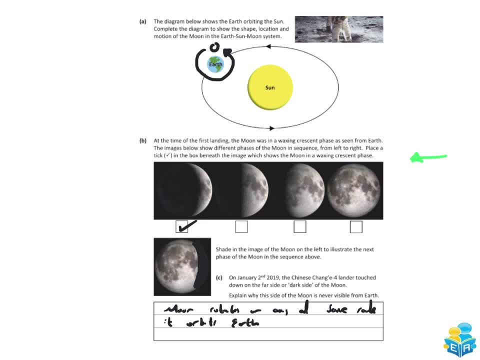 orbits the moon or it orbits the earth, okay, so it's much the same rate as when it's rotating on its axis, as it is orbiting around the earth. so that's why we never see the dark side of the moon. you actually needed both of those points there. for full marks. you need to mention the axes and 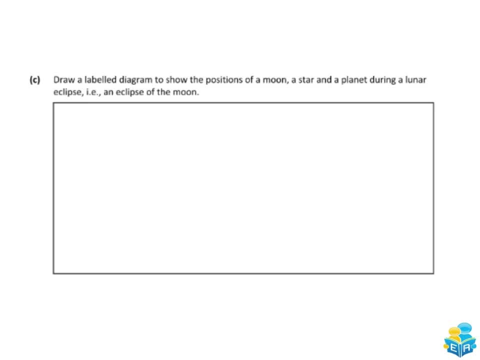 you need to mention the orbit around the earth as well. draw a label diagram to show the positions of a moon, a star and a planet during a lunar eclipse. so any clips of the moon. so this is one we see earlier on. so there's your sun, we have our earth, our moon. 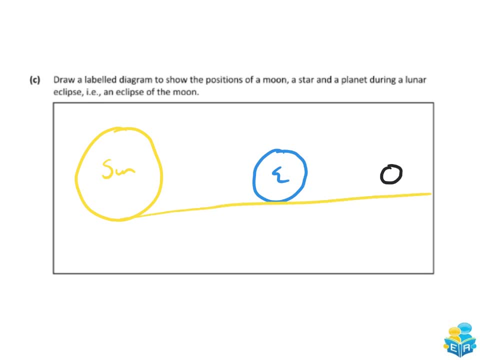 is going to be over here. it doesn't matter where the sunlight is trying to come from. it's going to be blocked off by the earth. okay, we'll have our umber region in here, we'll have our penumbra region in here, and the shadow of the earth is going to be cast onto the moon. 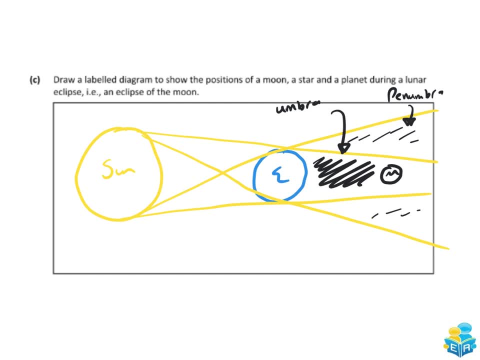 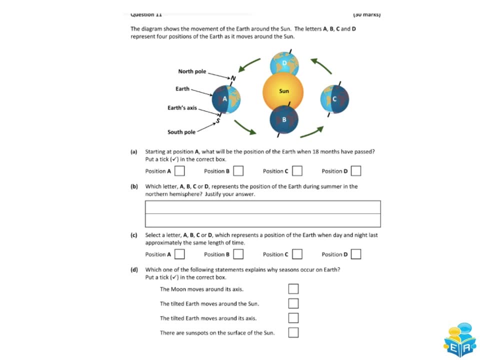 making it look like it has a shadow when it's going to appear more dark. okay, so that's the lunar eclipse and final question for today. the diagram shows the movement of the earth around the sun. the letters a, b, c and d represent four positions of the earth as it moves around the sun. starting at position a, what will be the position? 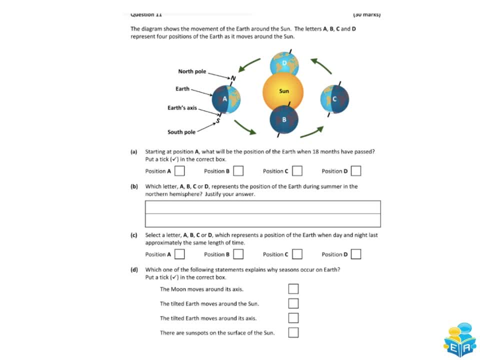 of the earth when 18 months have passed. so this happens once every 12 months. so this is going to be three months, three months, three months and three months. so in 12 months it's going to be right back to where it started. so in half of 12 months, in half a year, it would be over here at. 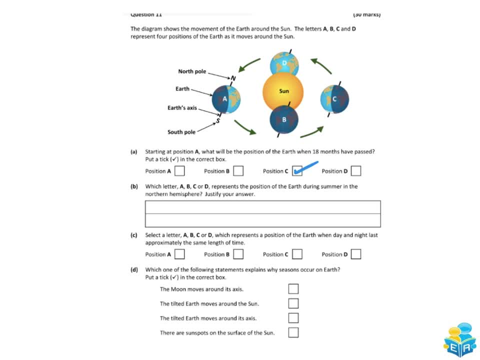 position c, which letter a, b, c or d represents the position of earth during summer in the northern hemisphere. so in the northern hemisphere we have to be tilted toward the sun. so that is going to be here. the northern hemisphere is tilted toward the sun here. so that's position a and we know that. 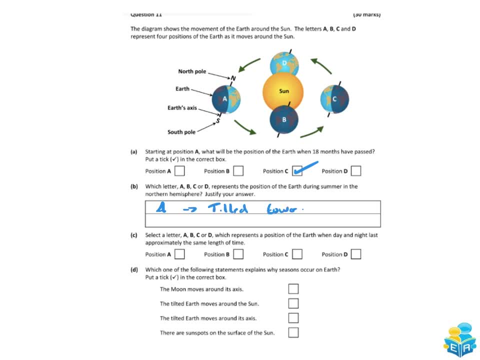 because it's tilted toward the sun. part c: select your letter- a, b, c or d, which represents the position of the earth when day and night last approximately the same length of time. so this is going to either be b or d, and then which one of the following statements explains: 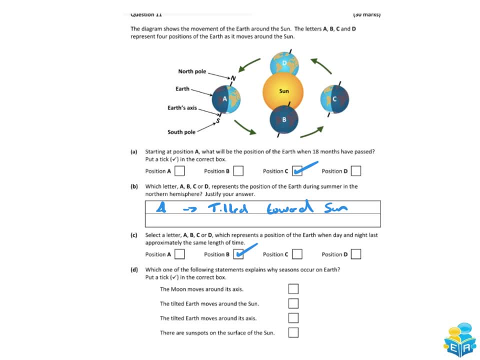 why seasons occur on earth. the moon moves around its axes, the tilted earth moves around the sun. the tilted earth moves around its axes, or there are sun spots on the surface of the sun. so this is the tilted earth moves around the sun, okay, which we came across earlier on. so that's a. 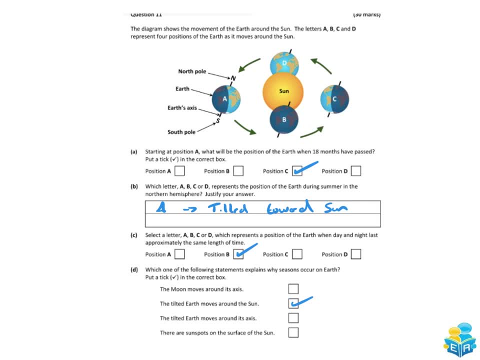 selection of questions which have come up on the phases of the moon, the seasons, the eclipses and the celestial objects. okay, they're very accessible questions. lots more questions have come up on these particular topics, so do make sure and go back and have a look at those as well. 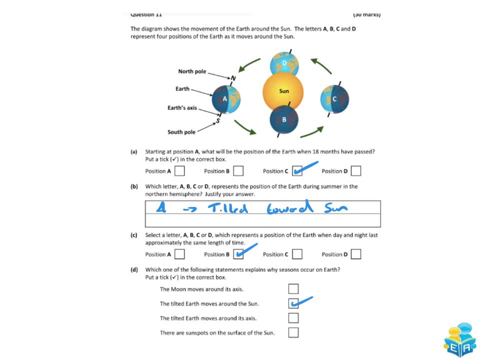 because they are very similar questions and there is a lot of repetition within them. now, just before we go, i do want to show you around the exam revision website where you can access more content, just like the content where we work through today. now, when you go to the exam, 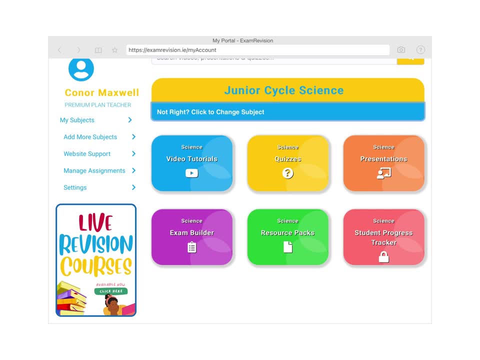 revision website, examrevisionie, and log in. you'll see that we've lots of different junior cycle subjects other than science as well. so we've business, geography, history, home ec, irish maths and science. all of them are laid out the exact same way. so we video tutorials. we've 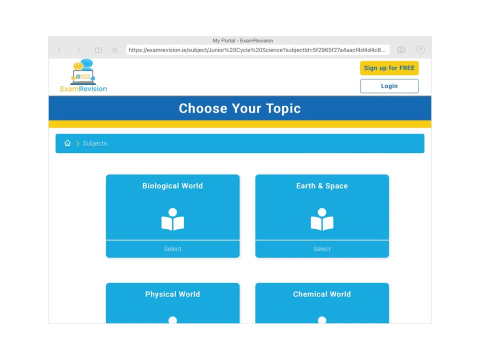 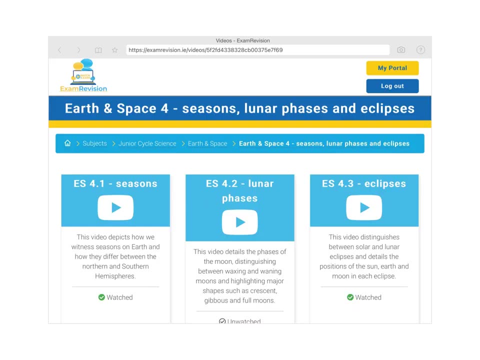 quizzes. we've presentations, an exam builder and a resource pack now within the video tutorials. today we were looking at earth and space, and one of the things we looked at was the seasons, the lunar phases and the eclipses. so you can click into the videos, watch back over all the contents. 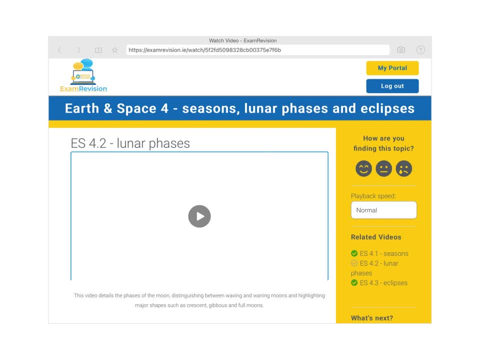 again, again and again, and again, at your own pace. you can change the playback speed to make it a little bit faster, a little bit slower, and there is related videos there for you to watch as well. now, if you go back to the home screen, we can see here not only do we have the videos, we have quizzes. 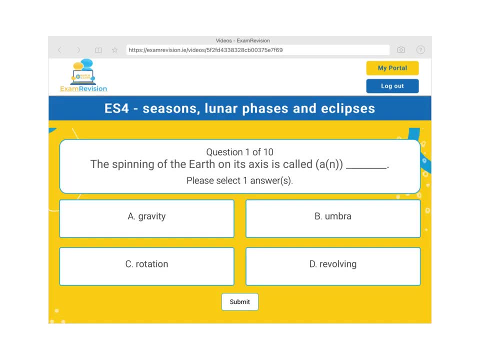 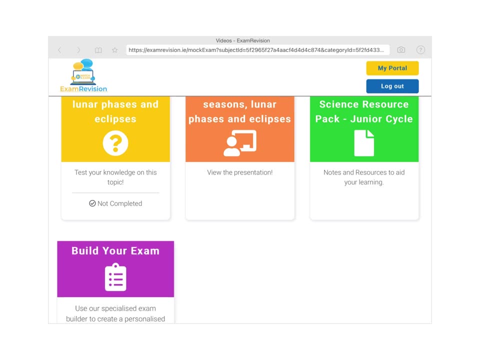 we have the eq quiz there: 10 questions which you can click through and test your knowledge. we do have a powerpoint presentation where you can get extra information, we have a resource pack which you can use in class, and we do have our exam builder as well. so again, not only are all the past state exam, 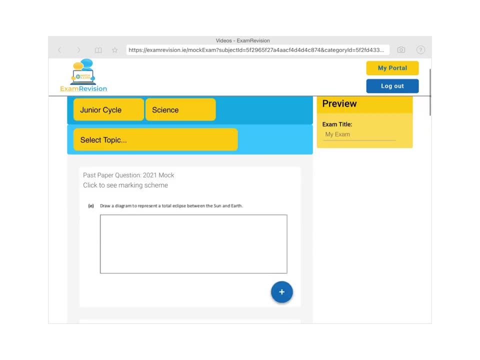 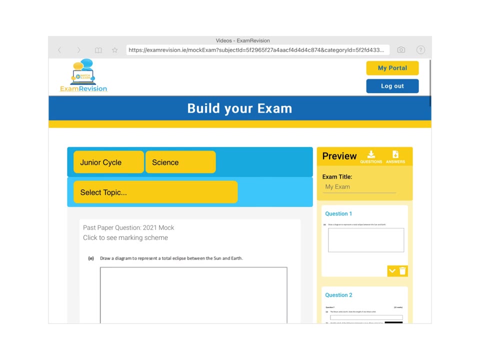 questions here. all the past mock questions are here as well, so you can have a look through those, pick whichever ones you want to add into your own exam, and when you go back up here to the top you have the option to download the questions and download the American schemes so you can test. 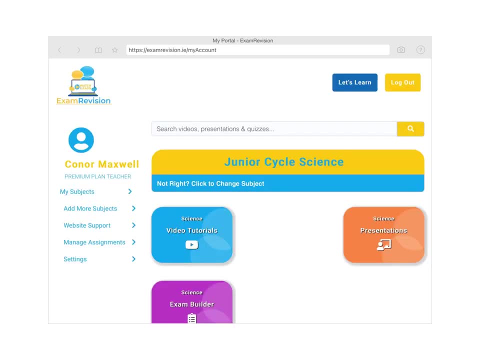 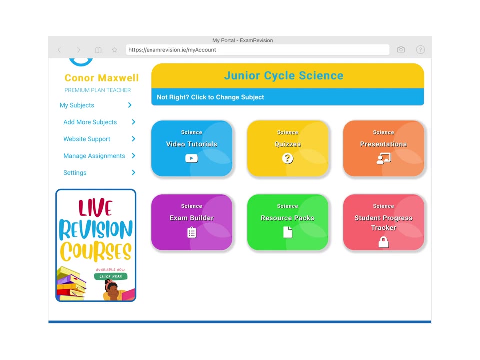 your knowledge as well. check out the exam revision website. we do also post some updates there about our live revision courses. so these are four hour revision courses, which happen usually during the midterm breaks, but also at Easter holidays and in May, June in the lead up to the exam as well. so it's an intensive.